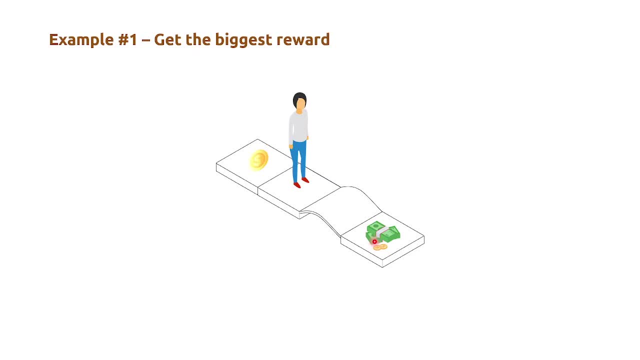 the agent will also receive a reward, assuming plenty. Okay, So the agent can either go to this state or go here. and then here I know The agent can go here or go here. So here, either state. So if the agent goes to either of the states, the game will end. 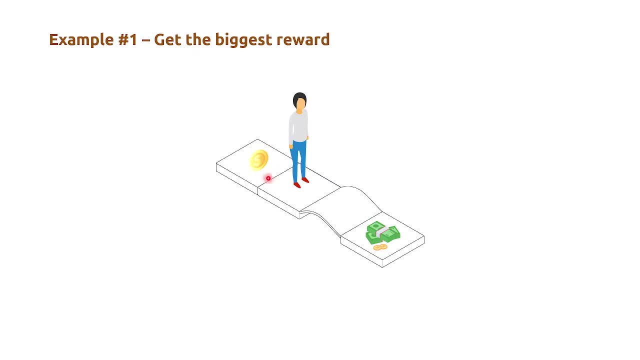 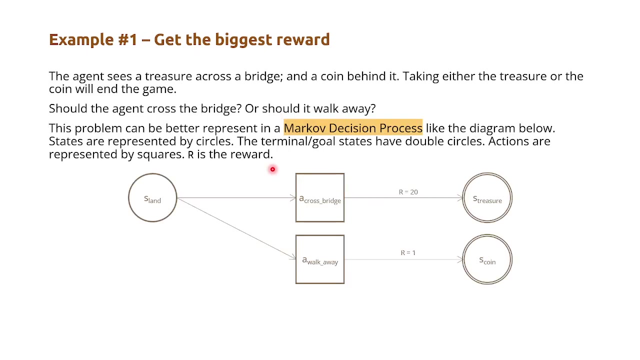 and the agent will get the reward that it has on that specific state. So this graphical representation of the world can also be represented in a markup decision process. So, as I have said, the agent sees a treasure across the bridge. So should the agent cross the bridge or should it walk away? So, as I have said earlier, 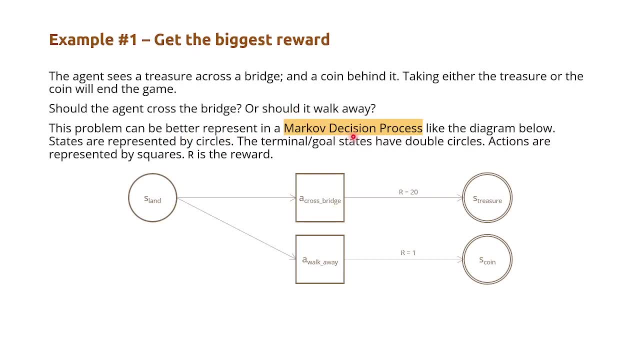 this problem can be better represented in a markup decision process like the diagram below. States are represented by circles, So this one, this is the state as land, And then this is another state as treasure and as coin, The terminal or goal states have. 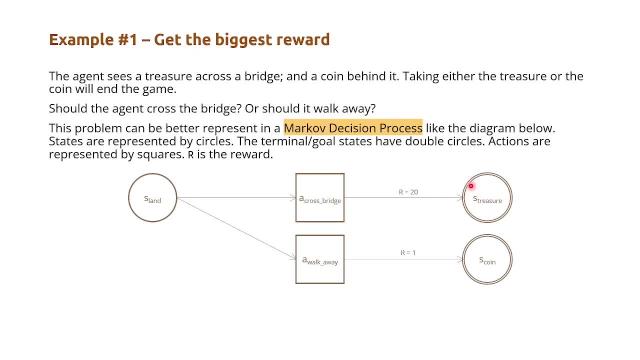 double circles. So this means that the agent can walk away from the treasure. So this is a terminal or goal state. This is also a terminal or goal state because both of these have double circles. The actions are represented by squares. This is an action. This is an. 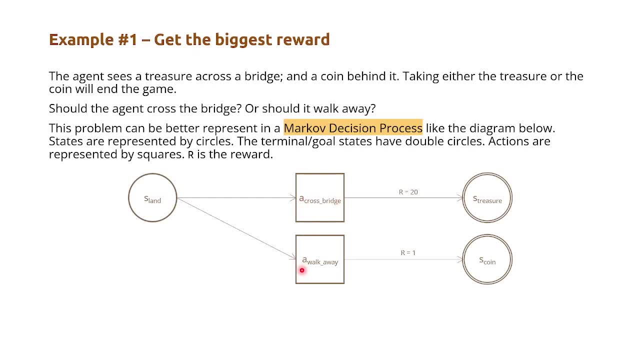 action. So the agent can either cross the bridge or the agent can walk away. R is the reward: taking that action. So if you go from- okay, So let's say that you are in state in a land- Then you decide to cross the bridge and you end up on the treasure. So that means 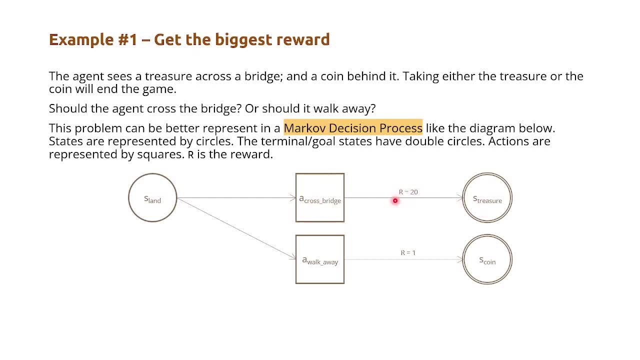 that the action of crossing the bridge to get the treasure will result in a reward of 20.. If you are in a land and you decide to walk away and then you get, and then you retrieve or you arrive at the coin state, that action will walking away, the action walking away. 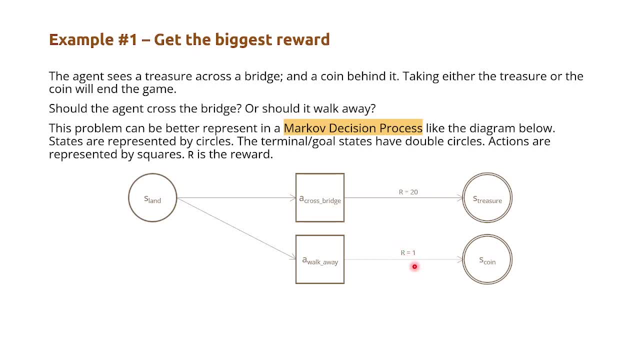 will grant you. Okay, So the first step is to get the reward of one. So now we want our agent to get the biggest reward, So we want to teach our agent to get the biggest reward. So, of course, 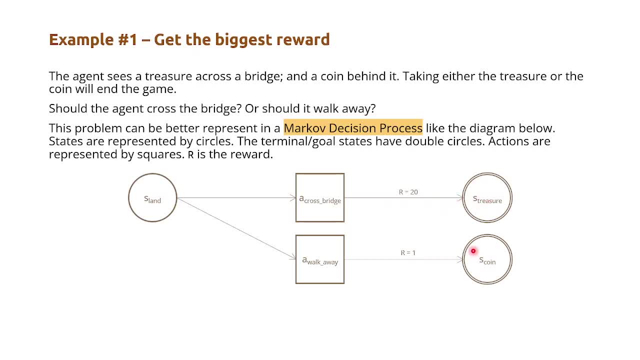 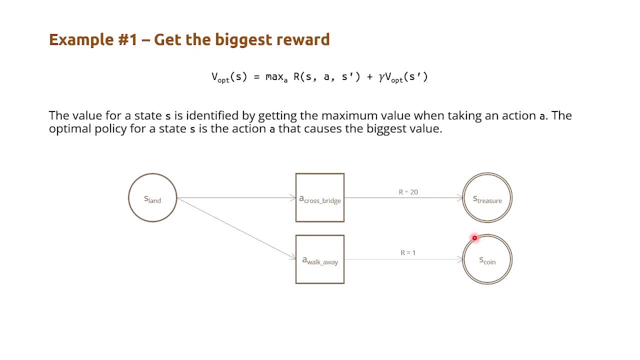 we want the agent to go to treasure instead of coin, right? So how do we make our agent do that? So actually, we can use the Bellman equation, Okay. Okay, we make some adjustments to the the equation. so now, as you can see, we have 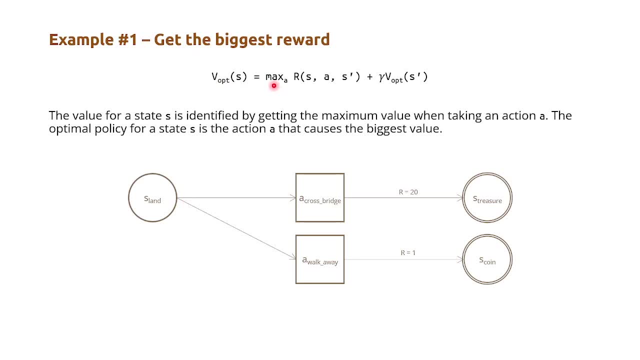 added the ax a for max action, discuss in a while. so, basically, the optimal, okay, the optimal value- repeat, the optimal value- of s is the action granting the maximum, okay, so the action granting the maximum utility or value of the of the succeeding state in this one. so we want, we want to identify which of these. 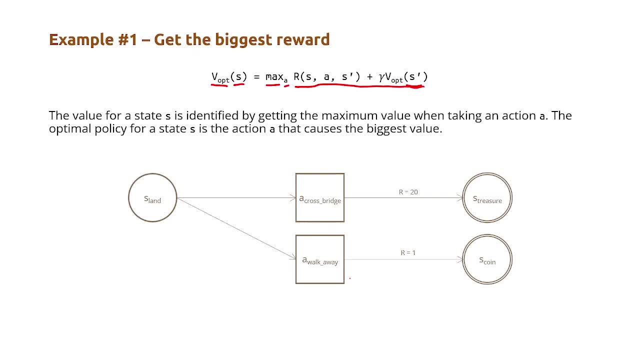 actions either cross, bridge or walk away, results in the maximized value. okay, okay, okay next time. so first we calculate the away for our phone. okay, so we replace the values. okay, so replace the value. so again we have the optimal of s is equal to max action. you are given the reward. 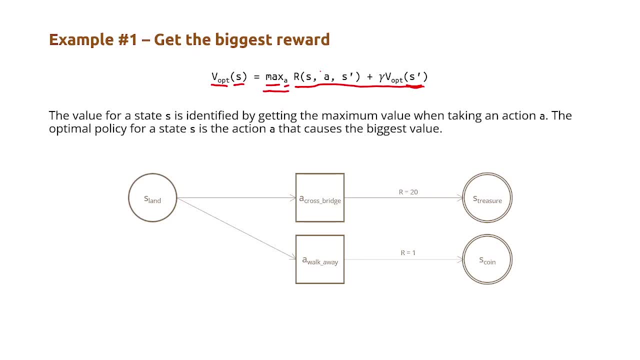 of in state s give ு were the optimal action of this estate as line. so that's why we plug in s land here. okay, so optimal value of s land is equal to max a r reward, reward of s land given the action. so we have two actions here: cross bridge and walk away. 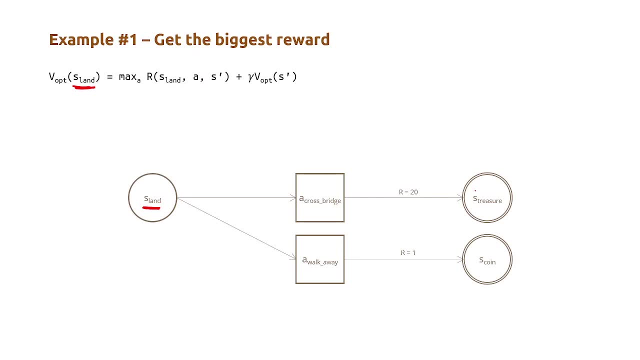 and then s prime. so the s prime of cross bridge is s treasure, the s prime of walk away is s coin plus our discount factor multiplied by the optimal value of s prime. okay, next, next side. so we just okay. now we calculate the values of each action of the state. okay, we calculate the value of each. 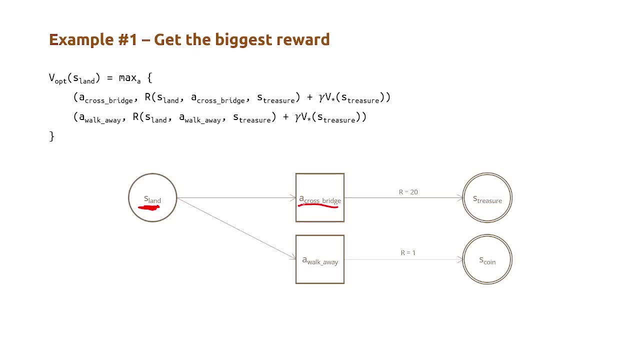 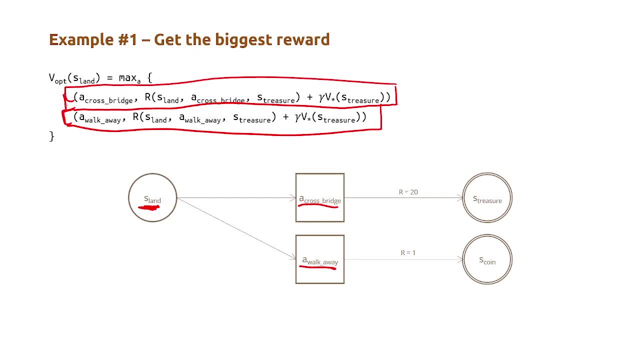 so i want you to focus on this one first. okay, focus on this first equation. okay. so the value of s land when performing action cross bridge is the reward of the reward of s land performing act, performing cross bridge, transitioning to s treasure, plus our discount factor multiplied by this is the opt. 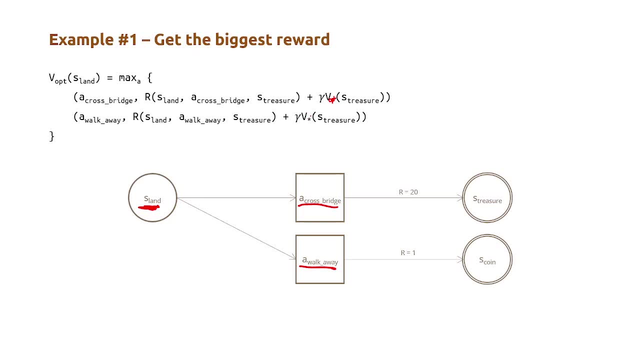 the optimal value of treasure. okay, so if you take a look, the reward of r s land cross bridge treasure is 20, right? so, uh, okay, i'll just write here this will be 20.. our gamma, so let's assume, assume um discount factor is 0.9, okay? 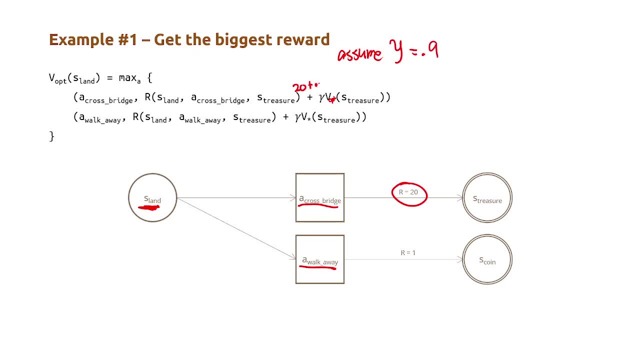 this will be 20.. our gamma, so let's assume um discount factor- is 0.9. okay, so gamma will be 0.9 plus. so gamma will be 0.9 plus 0.9 times, uh, the value of treasure. so, since this, 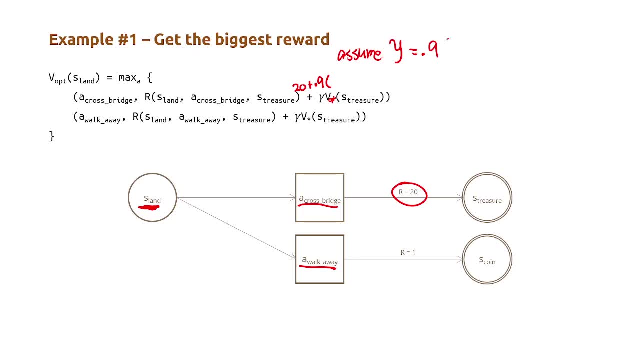 0.9 times uh the value of treasure. so, since this, 0.9 times uh the value of treasure. so, since this is uh the goal state, the value its value will be, is uh the goal state the value its value will be. is uh the goal state the value, its value will be zero. 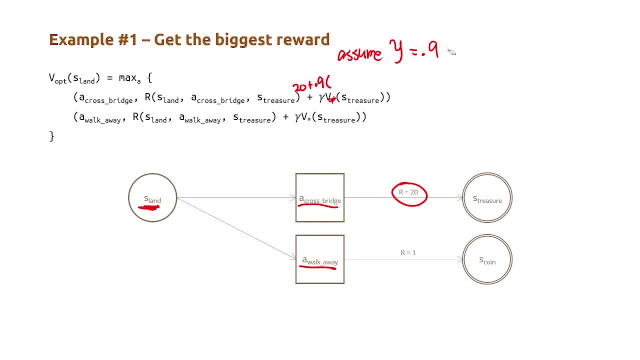 zero, zero- oh, not there- and zero, okay. so next, uh, let's take a look at the second equation, so the value and zero. okay. so next, uh, let's take a look at the second equation. so the value and zero. okay, so next, uh, let's take a look at the second equation, so the value of s land. when performing the, 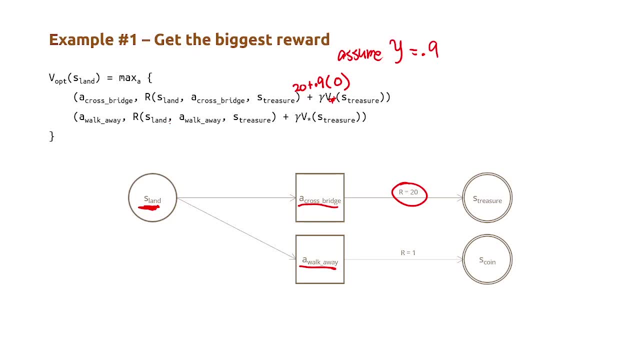 of s land when performing the of s land when performing the action. walk away is action, walk away is action. walk away is the reward of s land. walk away s pressure, the reward of s land. walk away s pressure. the reward of s land, walk away s pressure. this is not a search, this is s coin. 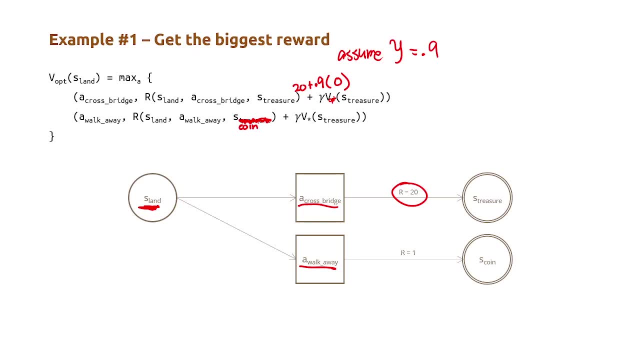 this is not a search. this is s coin. this is not a search. this is s coin. apologies, apologies, apologies, this is s coin. okay, this is s coin. okay, this is s coin. okay, this is also. this is also. this is also this point, this point, this point: yeah, it's s coin because, well, we have no. 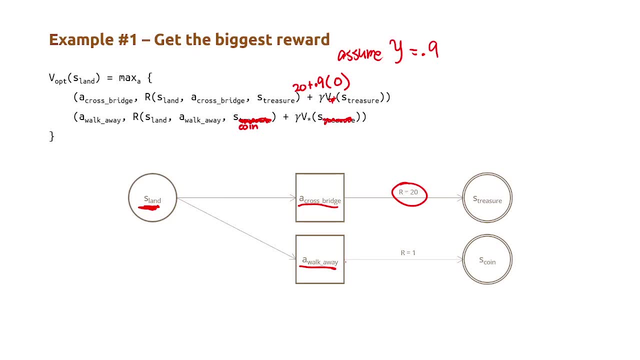 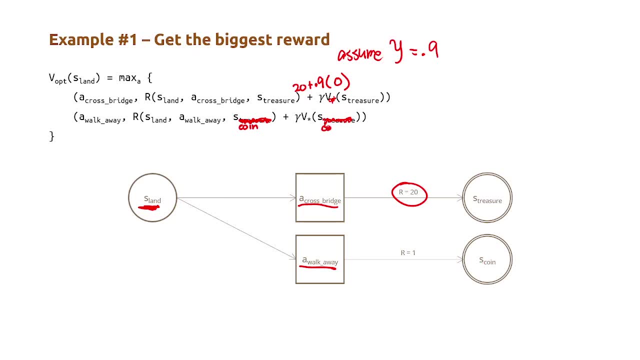 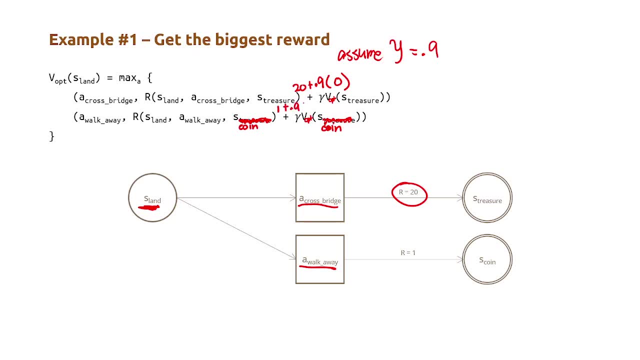 away s coin. it is away s coin. it is one plus point nine times one plus point nine times one plus point, nine times times the value of v opt of s coin. it is times the value of v opt of s coin. it is times the value of v opt of s coin. it is zero because it is the terminal state. 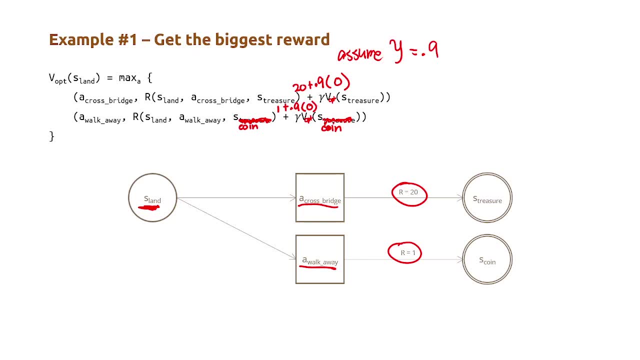 zero because it is the terminal state. zero because it is the terminal state. so if we proceed to be so, if we proceed to be so, if we proceed to be, next slide, you'll just see the same next slide. you'll just see the same next slide, you'll just see the same equation that i've written. 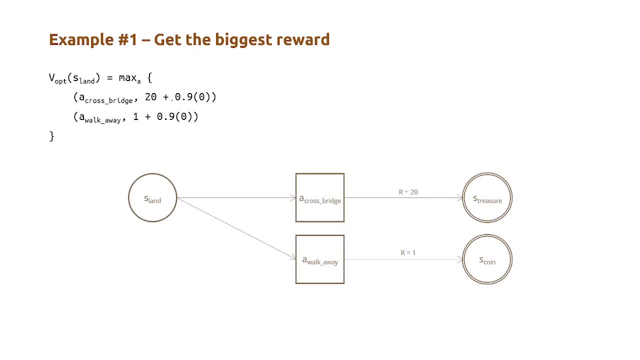 equation that i've written. equation that i've written: okay, so we have 20 plus okay, so we have 20 plus. okay, so we have 20 plus 0.9, right? 20 plus 0.9 times zero. 0.9 right? 20 plus 0.9 times zero. 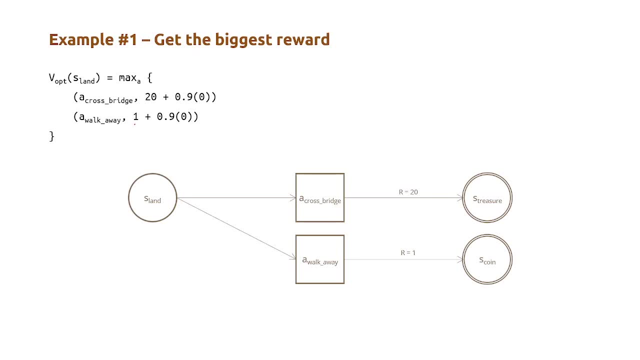 0.9 right, 20 plus 0.9 times zero. then, uh, when you walk away, you have. then, uh, when you walk away, you have. then, uh, when you walk away, you have one plus 0.9 times zero, one plus 0.9 times zero. 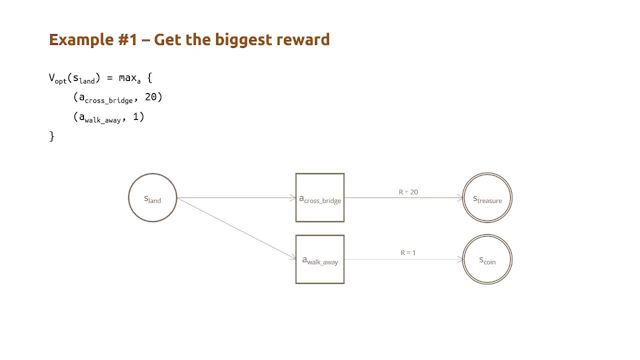 one plus 0.9 times zero. so next, so next, so next, okay, okay, okay, so so. so, now that we have calculated the values, now that we have calculated the values, now that we have calculated the values of of of s land, when performing each action cross, 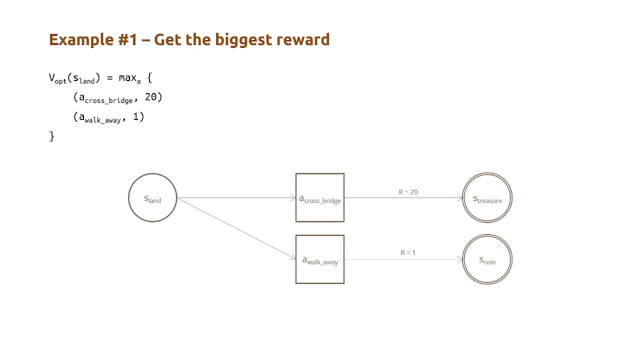 s land when performing each action cross s land. when performing each action, cross bridge and walk away. bridge and walk away. bridge and walk away. which is the maximum? is it 20 or 1? okay, which is the maximum? is it 20 or 1? okay, which is the maximum? is it 20 or 1? okay? again, so, which is the maximum value? is it? 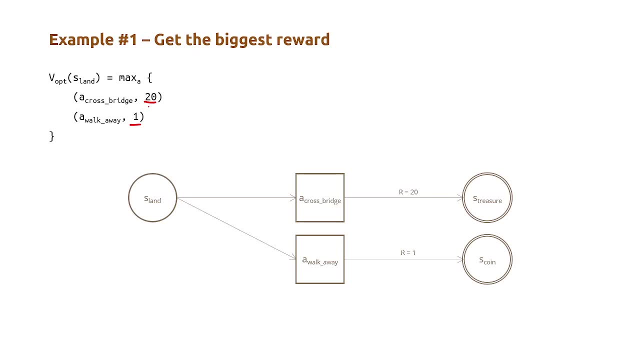 again. so which is the maximum value? is it again? so which is the maximum value? is it 20 or 1? 20 or 1? 20 or 1? it's 20, right, so it's 20, right, so it's 20, right. so the value of? 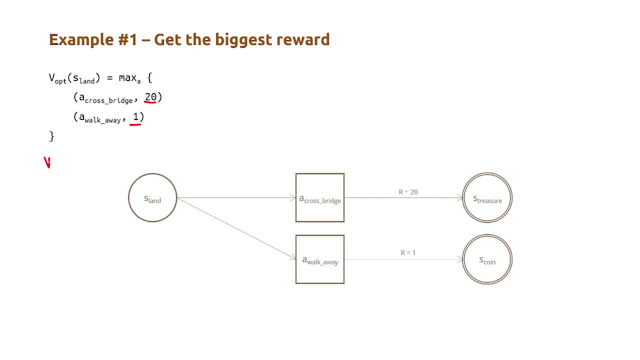 the value of the value of uh optimal value of s land will be: the optimal value of s land will be: the optimal value of s land will be the opt of s land, the opt of s land, the opt of s land will be 20.. will be 20.. 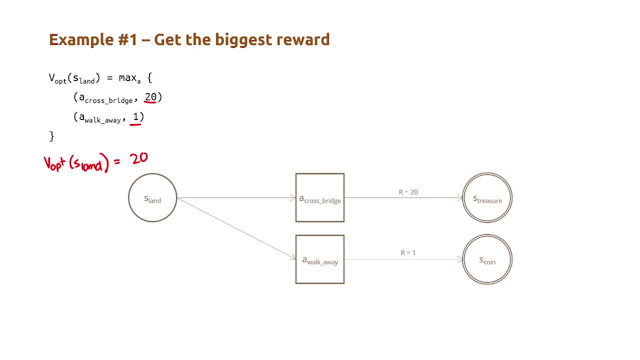 will be 20.. yeah, okay, so that's just that's just how. yeah, okay, so that's just that's just how. yeah, okay. so that's just that's just how simple it is simple, it is simple, it is okay. and then, since crossing the bridge, 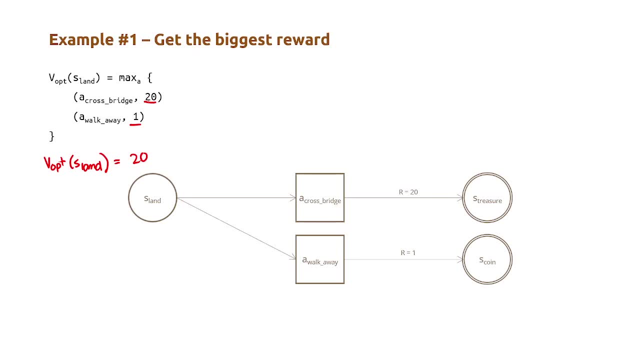 okay. and then, since crossing the bridge, okay, and then, since crossing the bridge, the action of crossing the bridge, the action of crossing the bridge, the action of crossing the bridge, is what gives the maximum value, is what gives the maximum value, is what gives the maximum value, then the optimal policy. 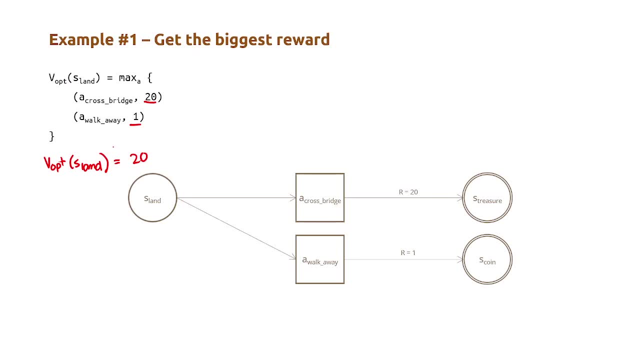 then the optimal policy, then the optimal policy of the uh the optimal policy, uh, when you of the uh, the optimal policy, uh, when you of the uh, the optimal policy, uh, when you are in s land, are in s land, are in s land, is to cross the bridge. okay, 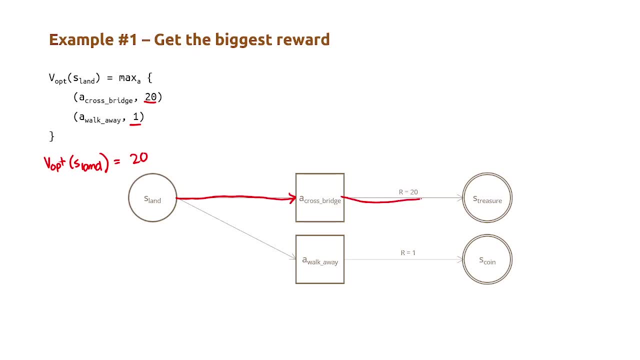 is to cross the bridge. okay, is to cross the bridge, okay. so the optimal policy is to cross the, so the optimal policy is to cross the bridge. next, next example: okay, now we have updated. okay, now we have updated. okay, now we have updated our world. so, in this example, 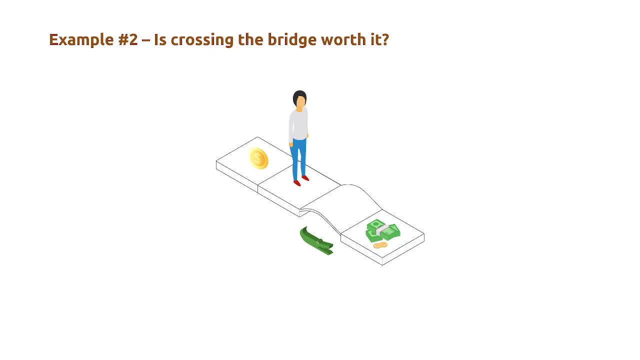 our world. so in this example, our world, so in this example, we have: okay, we still have two, three, we. we have. okay, we still have two, three, we we have. okay, we still have two, three. we now have three states, now have three states, now have three states, all right, 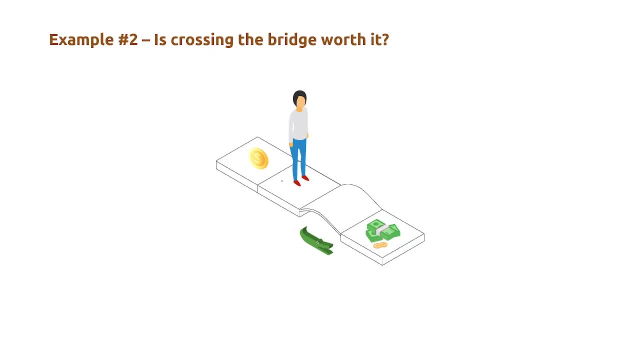 all right, all right, now we have four, so we have this state. now we have four, so we have this state. now we have four, so we have this state, our s land, so this is s land, our s land, so this is s land, our s land, so this is s land, this is s coin. 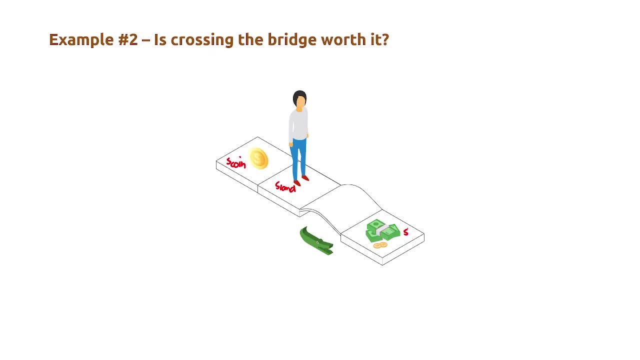 this is s coin. this is s coin s coin. this is s s coin. this is s s coin. this is s um treasure. also we have. we have added another. also we have. we have added another, also we have. we have added another state. we have s crocodile. 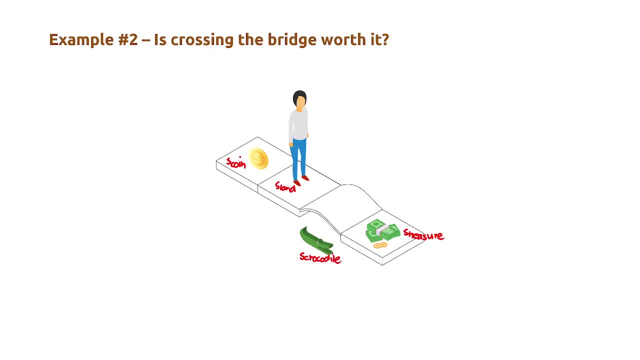 so what chain? so what chain? so what chain in this world? so, aside from adding a new in this world, so aside from adding a new in this world, so aside from adding a new state s crocodile state s crocodile state s crocodile, this bridge can also break, so let's just 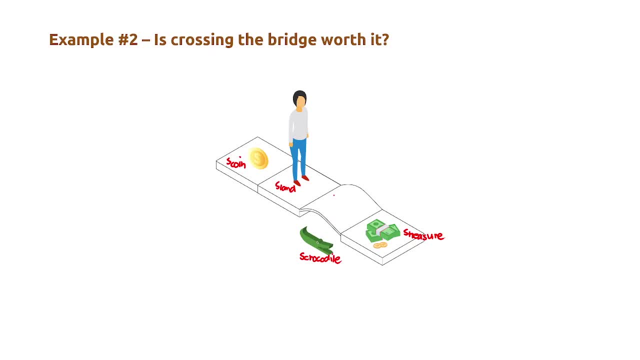 this bridge can also break. so let's just this bridge can also break. so let's just assume that this bridge is very old. assume that this bridge is very old. assume that this bridge is very old, and because it is very old, it has a. and because it is very old, it has a. 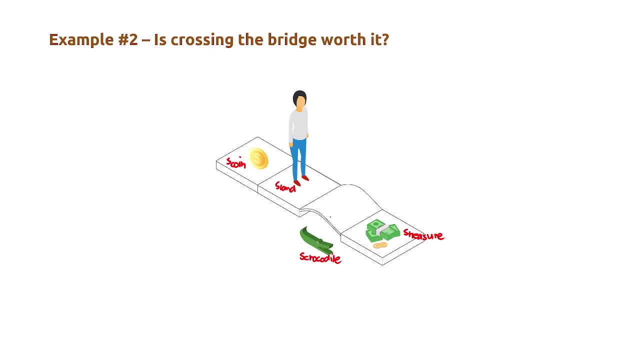 and because it is very old, it has a chance of breaking. when the agent will chance of breaking, when the agent will chance of breaking, when the agent will step on it, step on it, step on it. so if the agent steps on the bridge, and so if the agent steps on the bridge and 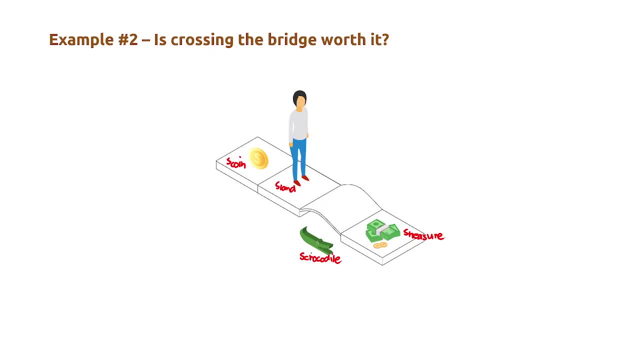 so if the agent steps on the bridge and it breaks, it breaks, it breaks, then the agent will fall to a crocodile, then the agent will fall to a crocodile, then the agent will fall to a crocodile. when the agent falls into a crocodile, a 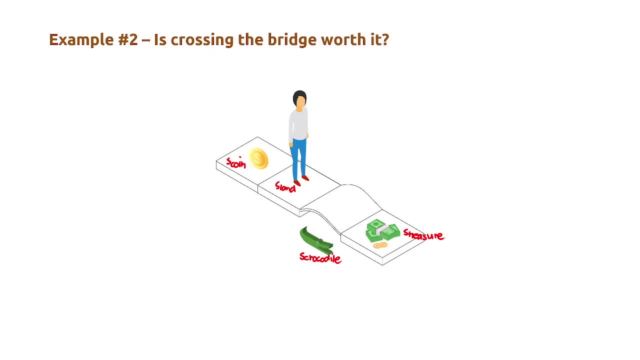 when the agent falls into a crocodile: a when the agent falls into a crocodile, a negative reward, negative reward, negative reward- will be given. or the agent will be will be given, or the agent will be will be given, or the agent will be punished, punished. punished, however, if the agent 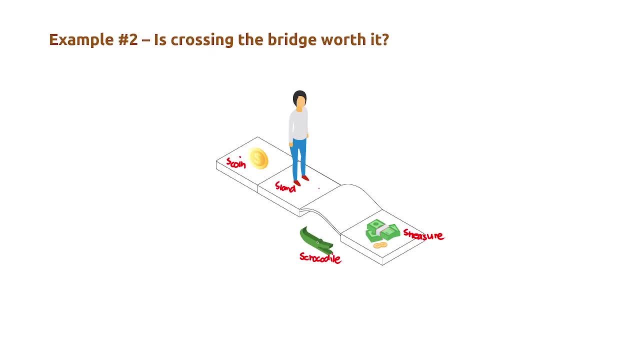 however, if the agent, however, if the agent successfully, successfully, successfully, um, um, um. if the agent successfully crosses the, if the agent successfully crosses the, if the agent successfully crosses the bridge, bridge, bridge, then the agent will get the treasure, then the agent will get the treasure, then the agent will get the treasure. so, um. 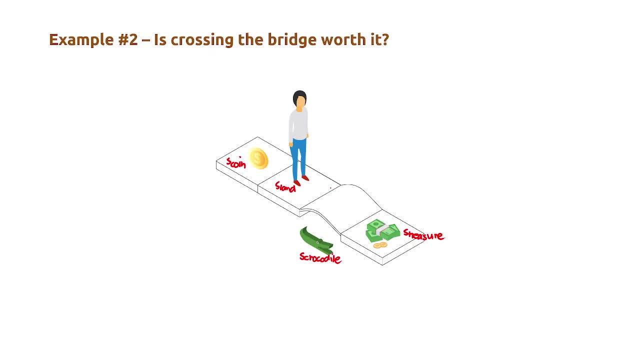 so, um, so, um, okay, so, the probability of. okay, so the probability of. okay, so, the probability of. so, the okay, so the probability of. so now we introduce probabilities. okay, so. so now we introduce probabilities. okay, so, so now we introduce probabilities. okay, so now we introduce probabilities in our 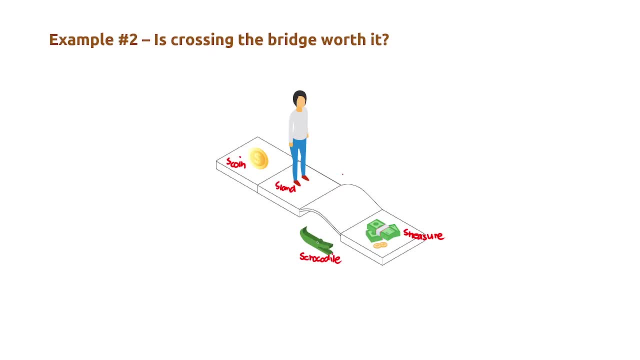 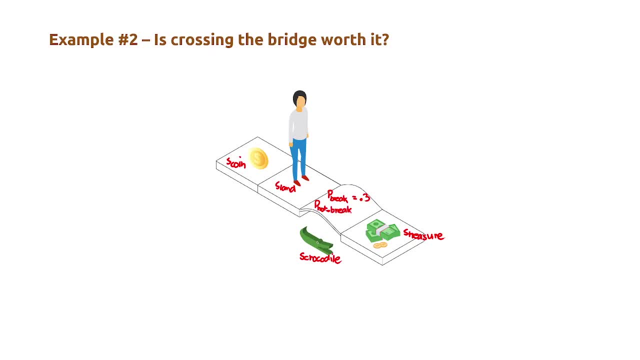 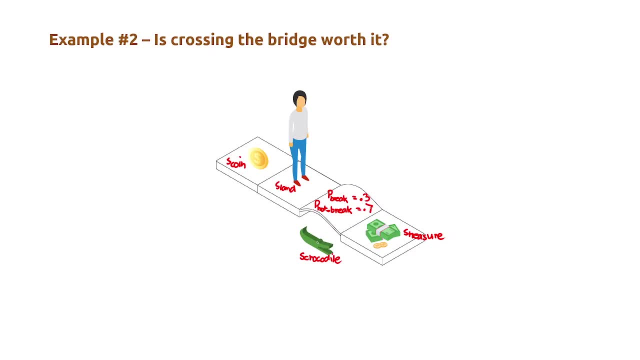 just means that this there is a 70. just means that this there is a 70, okay, there is a 70, okay, there is a 70, okay, there is a 70 success rate or 70 success rate, or 70 success rate or 70 chance that the agent will successfully. 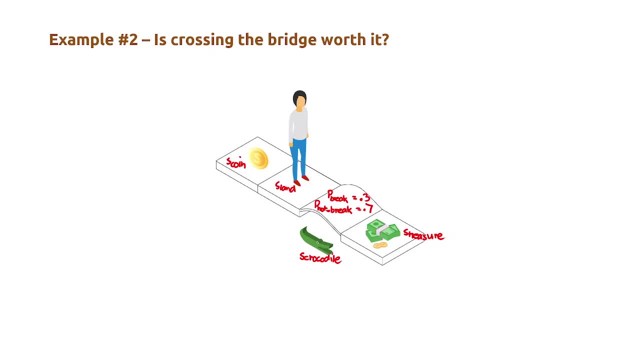 chance that the agent will successfully chance that the agent will successfully cross the bridge and get the pressure cross the bridge and get the pressure cross the bridge and get the pressure and there is a 30 chance and there is a 30 chance and there is a 30 chance that the agent will not. 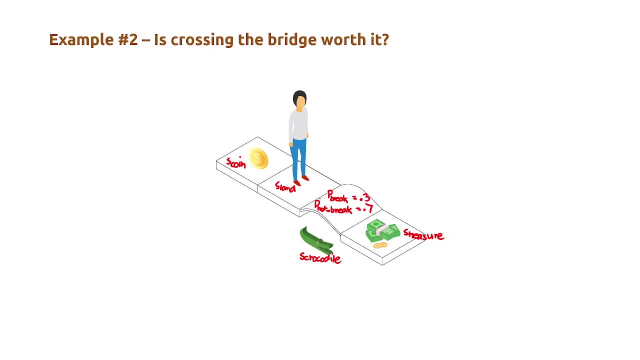 that the agent will not, that the agent will not get the pressure because um, because the get the pressure because um, because the get the pressure because um, because the bridge will break, bridge will break, bridge will break and the agent will fall into our and the agent will fall into our. 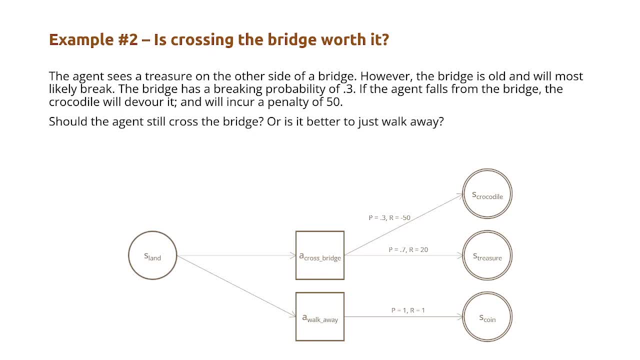 and the agent will fall into our crocodile. so we can represent it in crocodile. so we can represent it in crocodile. so we can represent it in another mark of decision process. another mark of decision process, another mark of decision process. all right, so i just added this one. 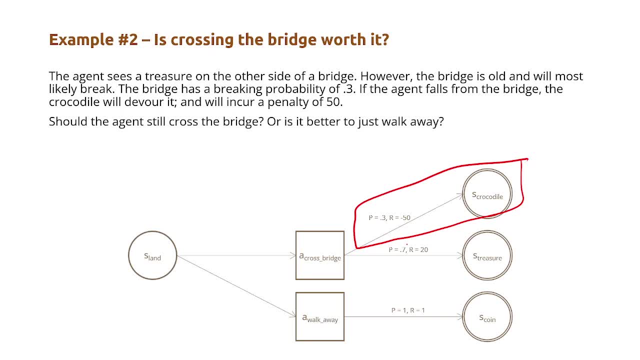 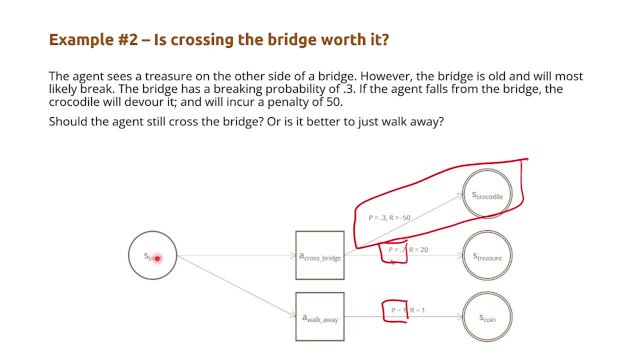 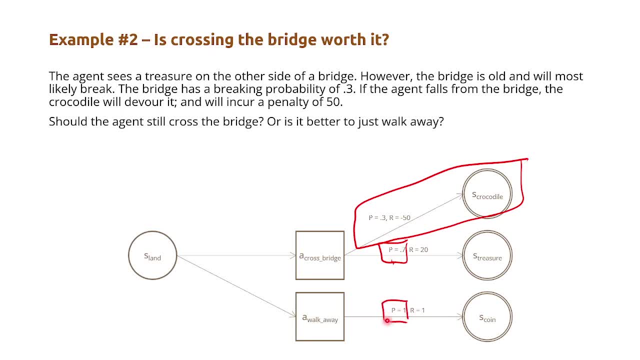 slan is one. slan is one meaning you have there's a 100 chance. meaning you have there's a 100 chance. meaning you have there's a 100 chance that you will successfully get the coin, that you will successfully get the coin, that you will successfully get the coin when you walk away. however, 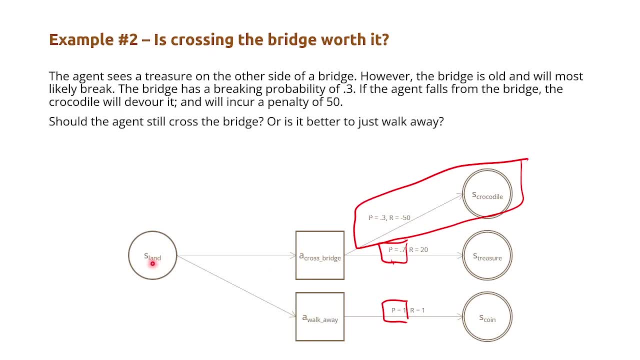 when you walk away. however, when you walk away, however, when, if you look at the top, if you when. if you look at the top, if you when. if you look at the top, if you decide, or if the agent decides to cross, decide, or if the agent decides to cross. 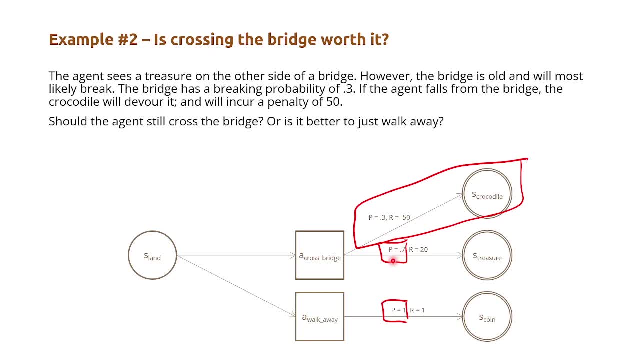 decide, or if the agent decides to cross the bridge, the bridge, the bridge. there is a 0.7 probability that there is a 0.7 probability that there is a 0.7 probability that, when crossing the bridge, the. when crossing the bridge, the. 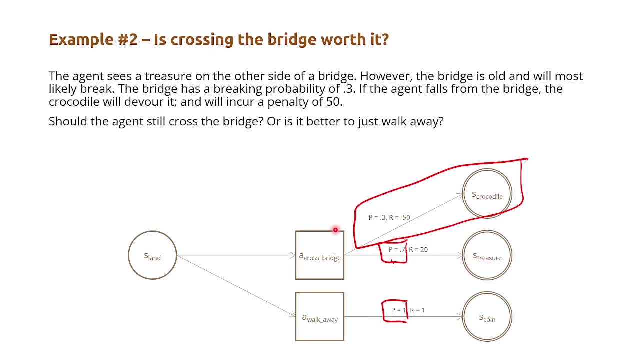 when crossing the bridge, the? um the agent will go to the treasure. um the agent will go to the treasure. um the agent will go to the treasure. there's also a 0.3 probability that the. there's also a 0.3 probability that the. 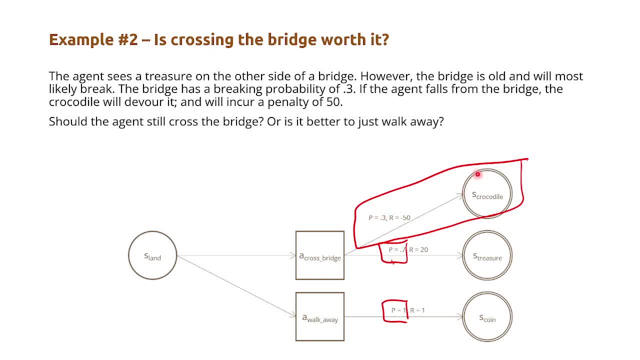 there's also a 0.3 probability that the agent will go to agent will go to agent. will go to the crocodile- the crocodile, the crocodile. also notice that the reward also notice that the reward also notice that the reward when going, when the agent falls into a 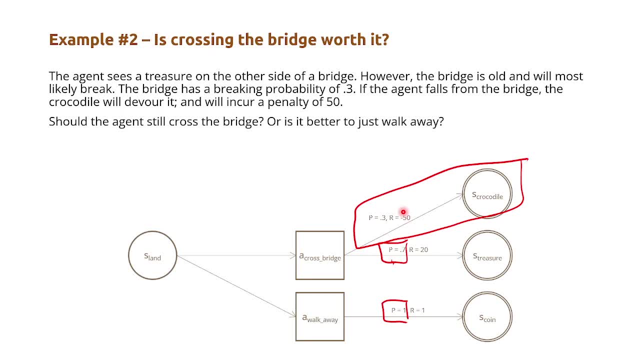 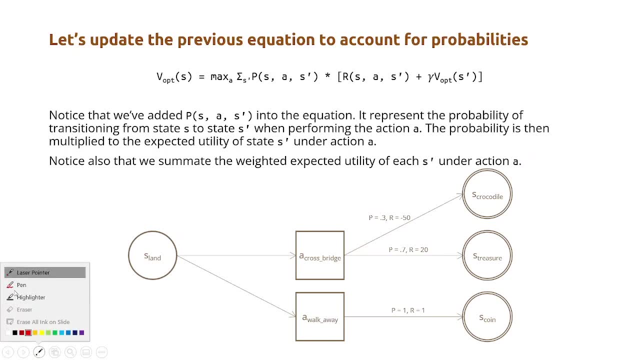 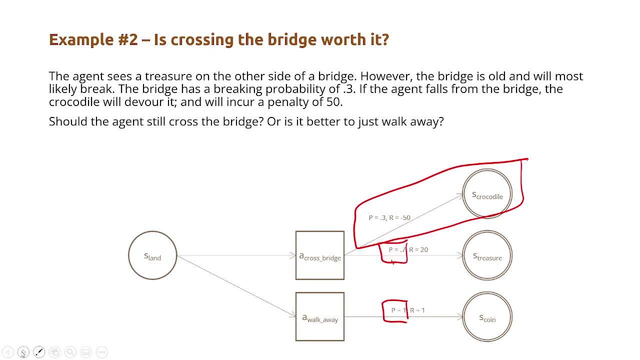 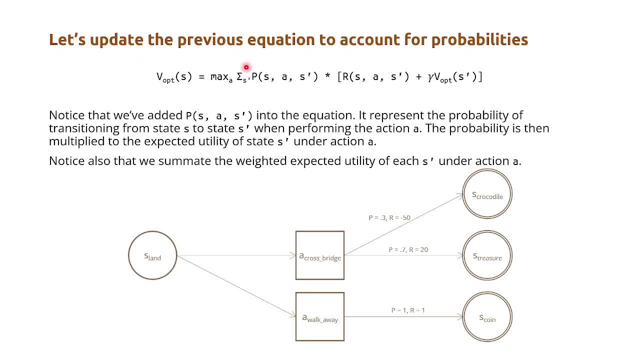 so let's update the previous equation to account for probabilities. account for probabilities. account for probabilities. so, uh, what i just added here is okay. what i just added here is this okay. what i just added here is this okay. what i just added here is this: probability: probability of um. 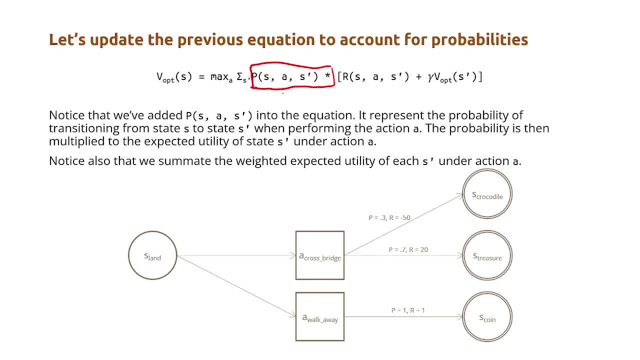 probability of um. probability of um transition. probability of um transition from s from s. from s to s prime. given the action a okay times to s prime. given the action a okay times to s prime. given the action a okay times, or multiplied by the. or multiplied by the. 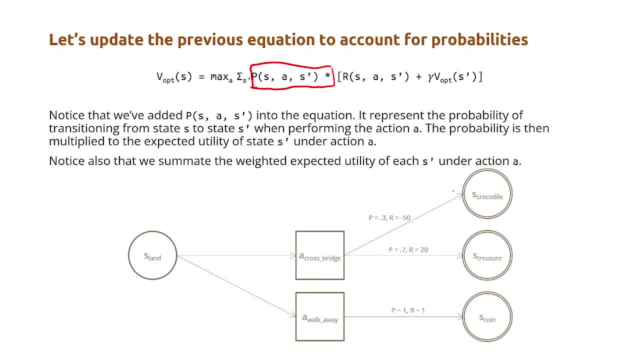 or multiplied by the expected reward from that action: okay, expected reward from that action. okay, expected reward from that action. okay. so let's just say, for example, uh, yes. so let's just say, for example, uh, yes. so let's just say, for example, uh yes, in the crocodile. so you have a 0.3. 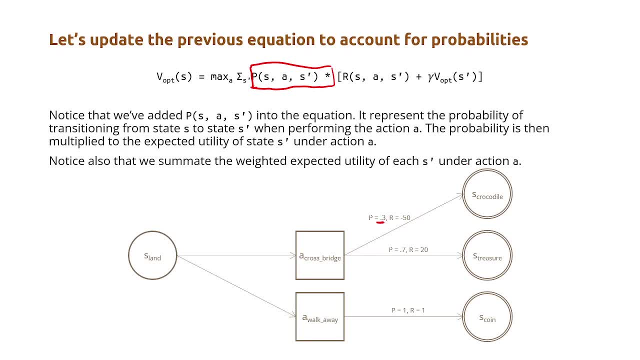 in the crocodile, so you have a 0.3 in the crocodile, so you have a 0.3 probability, right? so we just multiply probability. right? so we just multiply probability. right? so we just multiply 0.3, 0.3 times the expected. 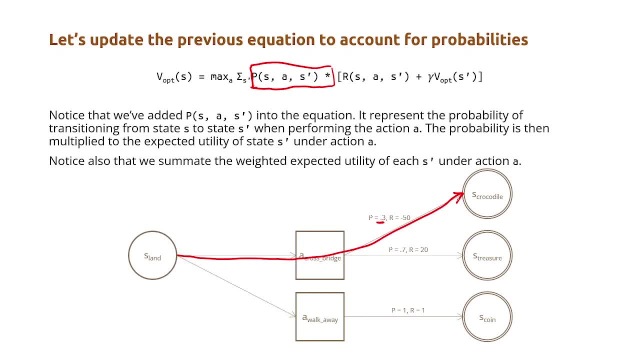 0.3, 0.3 times the expected, 0.3, 0.3 times the expected reward of this path, reward of this path, reward of this path. okay, another thing, we also multiply 0.7. okay, another thing, we also multiply 0.7. 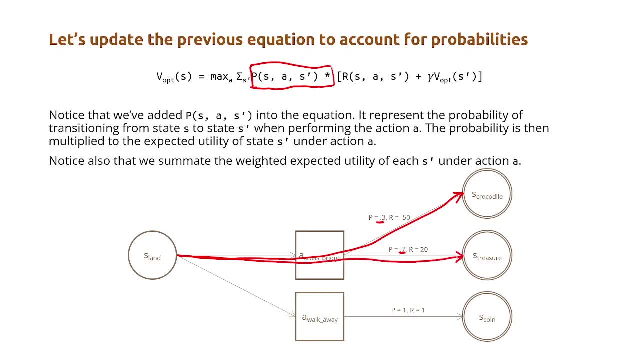 okay, another thing: we also multiply 0.7 to the expected reward of this path, to the expected reward of this path, to the expected reward of this path after we multiplied each. so this will, after we multiplied each, so this will after we multiplied each. so this will have, uh, different values. so now we have. 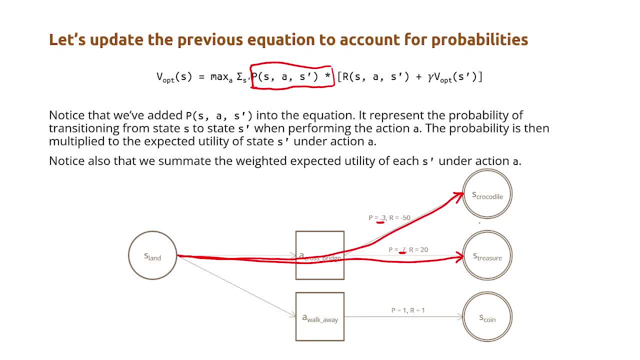 have uh different values. so now we have have uh different values. so now we have two values, two values, two values. we just add those two values. we just add those two values. we just add those two values afterwards. so this is why i have to make afterwards, so this is why i have to make. 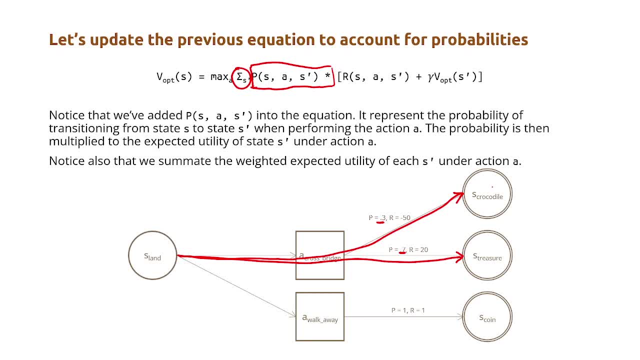 afterwards. so this is why i have to make this function, this function, this function: just add those two values, just add those two values. just add those two values under, under, under, okay, okay, okay, okay, under this action, under one action, okay, after adding those values, okay, after adding those values. 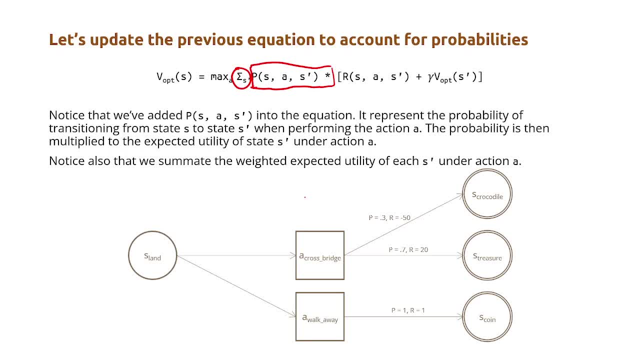 okay, after adding those values, that the resulting value or the submitted that the resulting value or the submitted that the resulting value or the submitted value will be the value. value will be the value. value will be the value of s land given uh when performing that of s land given uh when performing that. 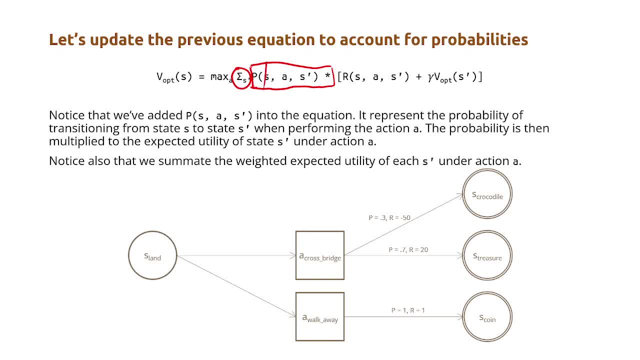 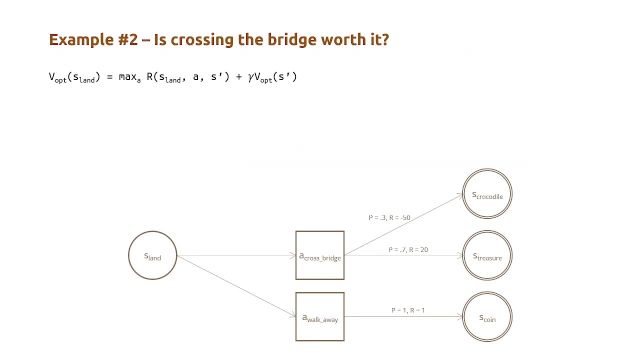 of s land given, uh, when performing that action cross bridge, action cross bridge, action cross bridge. okay, so, next slide. so our, of course, our equation, so our, of course, our equation, so our, of course, our equation: the optimal value of s land is equal to. the optimal value of s land is equal to. 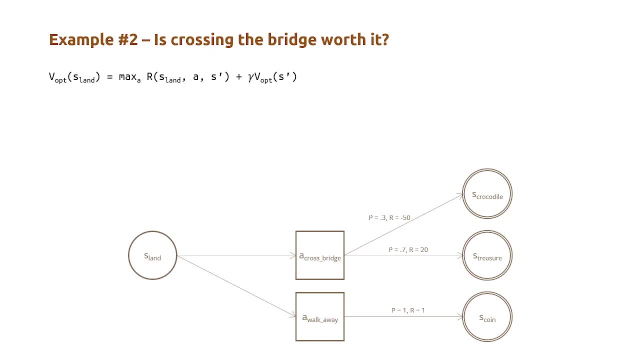 the optimal value of s land is equal to the maximum, the maximum, the maximum. okay, so this is lacking. sorry, you missed things. sorry you missed things, sorry you missed things. so we have max, a summation of. so we have max, a summation of. so we have max, a summation of prime. 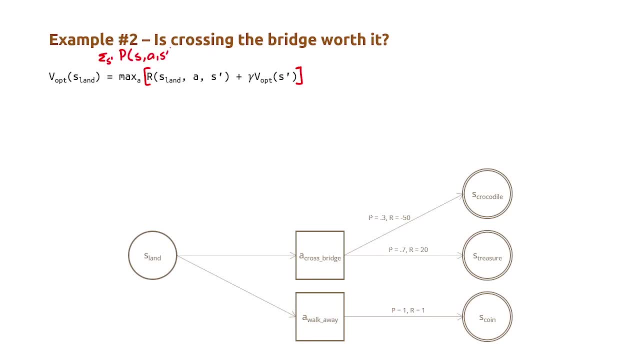 prime prime p p p s s s s s s prime times, s s prime times, s s prime times. okay, the edges, okay, the edges, okay, the edges times. this the one in brackets, okay, okay, okay, okay, it's something more exciting, it's something more exciting, it's something more exciting. so, yeah, so we first. 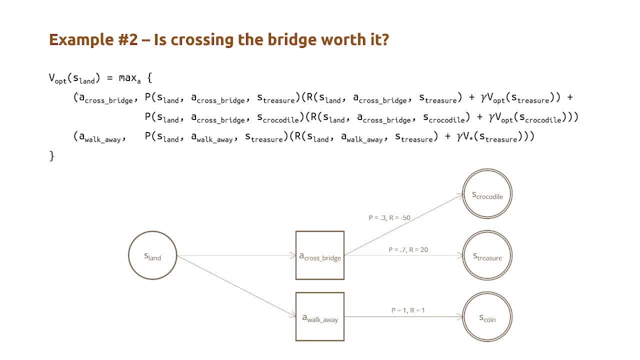 so yeah, so we first. so yeah, so we first um, um, um. okay, so the we have two different. okay, so the we have two different. okay, so the we have two different equations here, equations here, equations here. we have this equation, we have this. we have this equation, we have this. 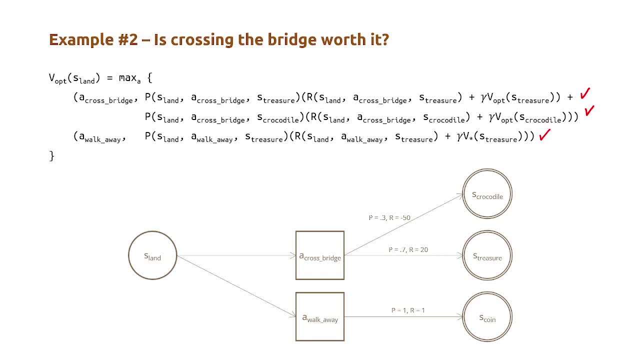 we have this equation, we have this equation, and then sort of this equation, equation, and then sort of this equation, equation, and then sort of this equation for each path: so we have this path right. equation for each path. so we have this path right. equation for each path. so we have this path right, we have this path, we also have this path. 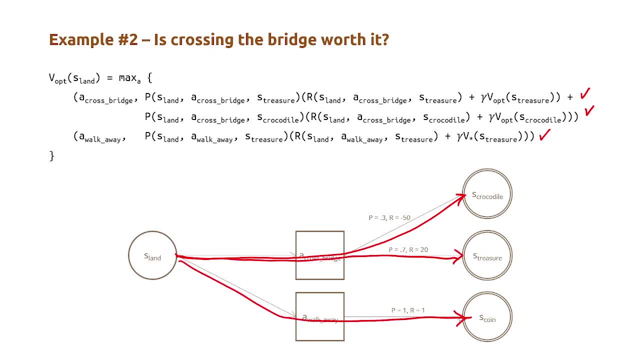 we have this path, we also have this path, we have this path, we also have this path, and we have this path and we have this path and we have this path. right, okay, so each path is represented, right, okay, so each path is represented, right, okay, so each path is represented by. 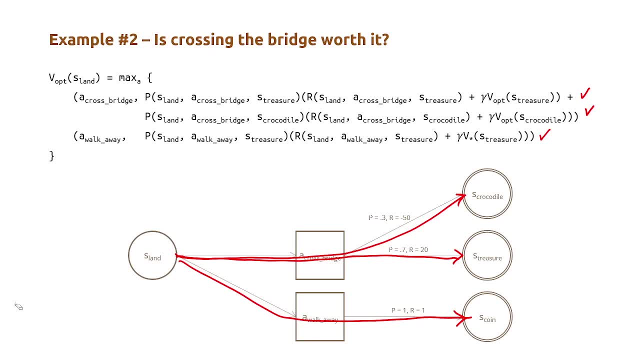 by by, different equations, different equations, different equations. okay. so different equations. okay. so different equations, okay. so it looks like that the first equation. it looks like that the first equation. it looks like that the first equation corresponds to, corresponds to, corresponds to this path. okay, this path okay. 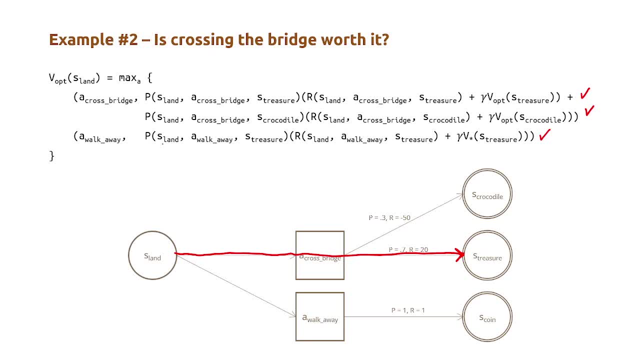 this path. okay, oops, oops, oops, okay, so the first equation corresponds to: okay, so the first equation corresponds to: okay, so the first equation corresponds to this path, this path, this path. so what is the probability of s land? so what is the probability of s land? 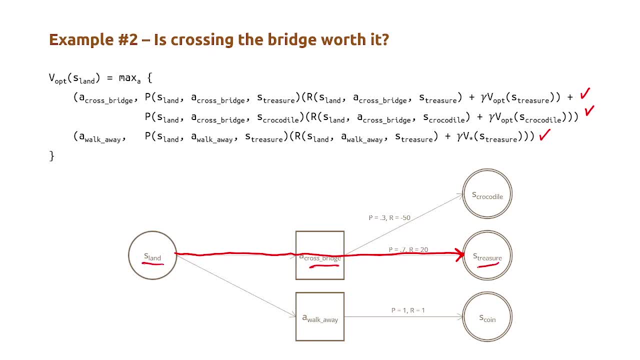 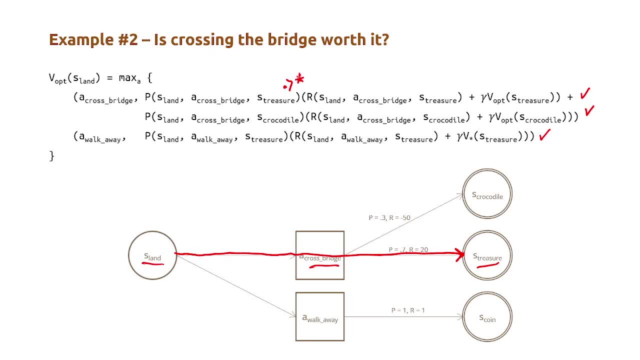 so we have. so we have 0.7, 0.7, 0.7 times times times. okay, So what is the reward of S-Land cross-bridge treasure? So the reward of S-Land cross-bridge treasure is 20, right? 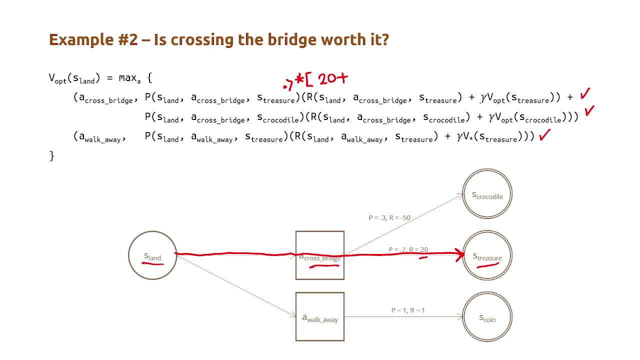 So 20 plus gamma, Our gamma is 0.9.. Let's just assume. Let's just assume that our gamma is 0.9.. And then what is the optimal value of treasure? Treasure. this is 0. because the optimal value of treasure is 0, because it is a growth state. 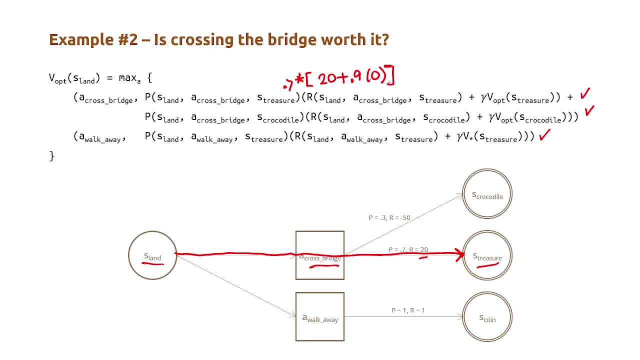 Times 0.. Okay, Next, You know what? I'll just write it here on the left side: 0.7 times 20 plus 0.9 times 0.. Okay, The next equation refers to this path. Refers to this path. 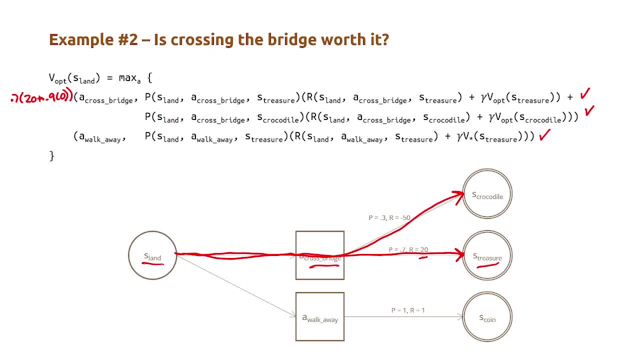 So what is the probability of S-Land cross-bridge crocodile? S-Land cross-bridge- S-Land cross-bridge- s-nand cross-bridge crocodile. it is 0.3 times reward of s-nand cross-bridge crocodile. 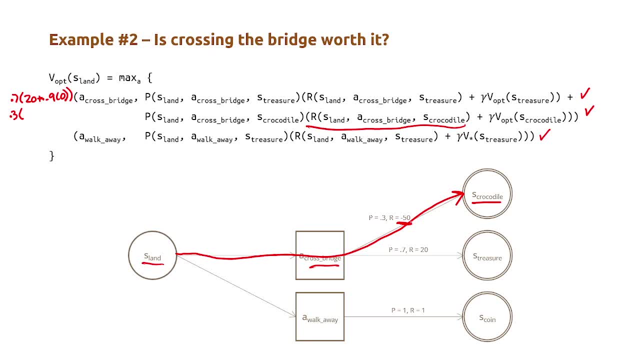 is negative 50. so negative 50 plus our gamma, which is 0.9 times the value of s crocodile. so the value of s crocodile is 0 because it is equal state. okay, good, after that we proceed with the calculation of the third path. okay, the third path. 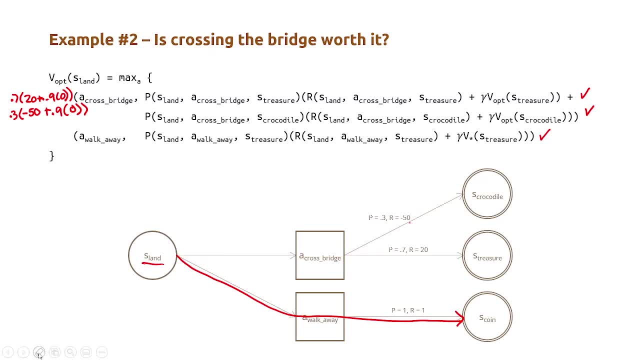 okay. third path refers to being in s-nand and then walking away, which is the point. so the probability of s-nand walk away coin is one right times reward of s-nand walk away coin reward is one. so 1 times 1 plus gamma, 0.9 times the value of s coin. the value of s coin. 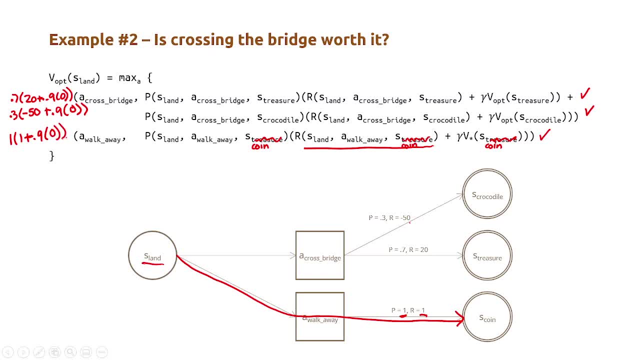 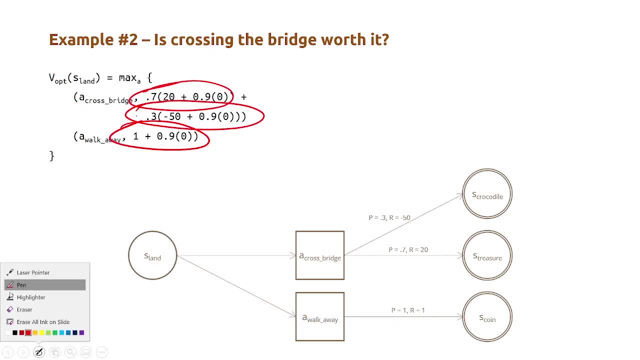 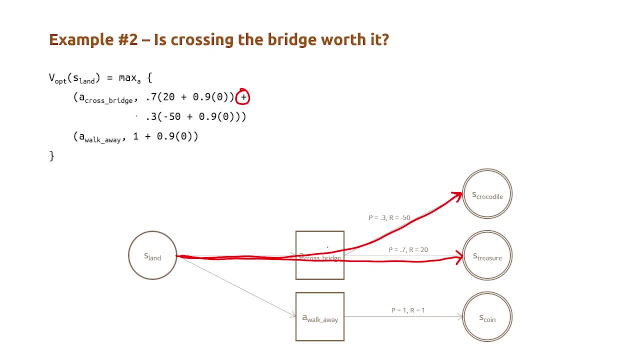 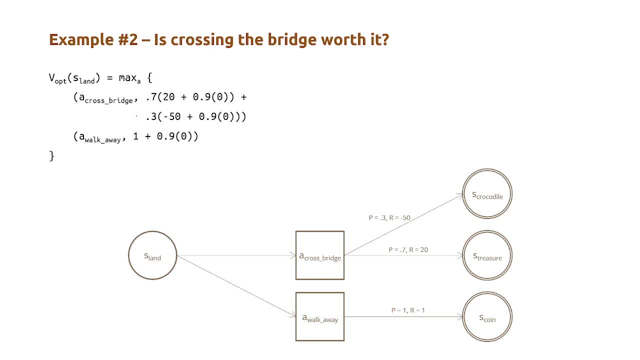 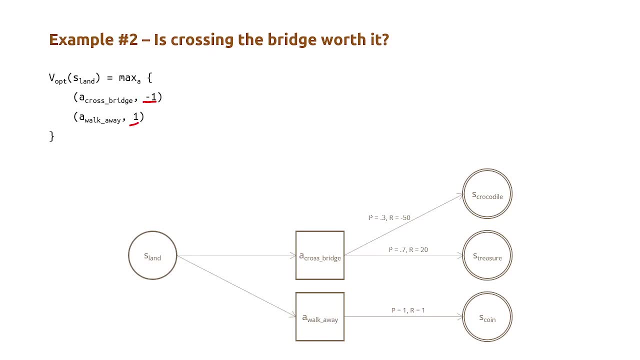 one. so, yeah, it's obvious, the, the maximum value is one right. so this tells us that if you are, if the agent is, in s-land, it is now better to walk away then to cross the bridge. so it's basically telling be the agent that it's not worth it. it's not worth it to cross the. 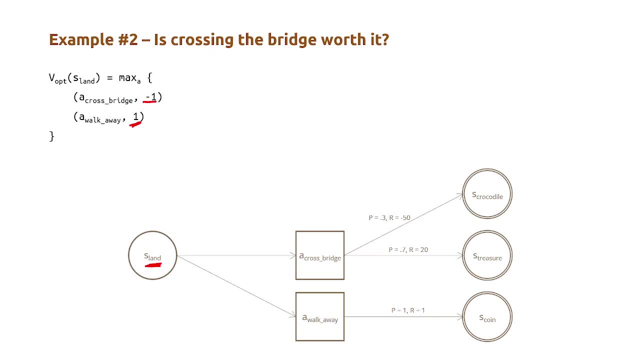 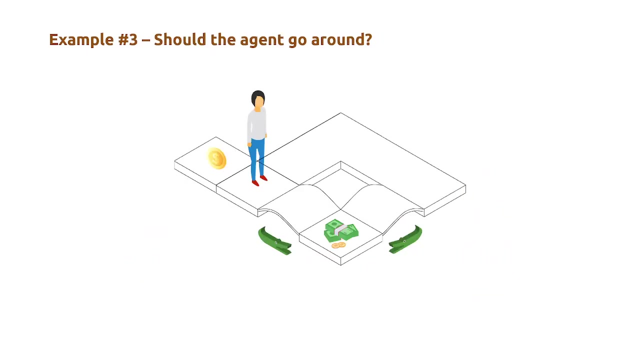 bridge, it's better to just walk away and get the you sure, regardless of one. ok, so this X, X, this x will be the path that our agent will take. so next example: so now we have, so now we have updated our um world right, so we have added this: 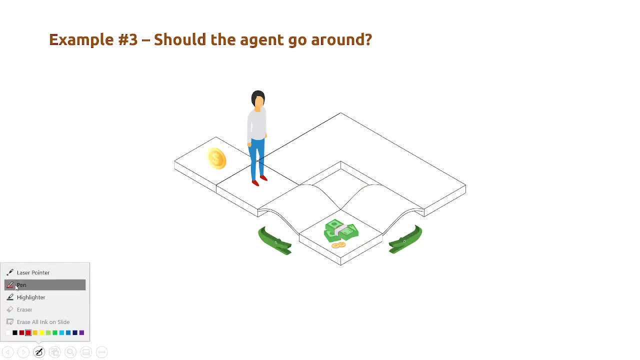 we have added this, so this one is another state. let's just call it s92. this one is another state, let's just call it s92. then this is still crocodile s crocodile. this is also s crocodile, so notice that we have two bridges now. this bridge has a um. 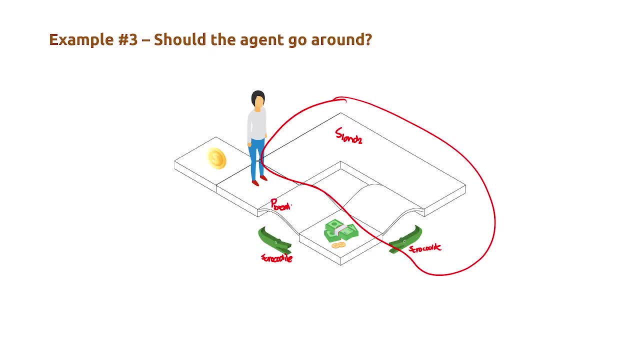 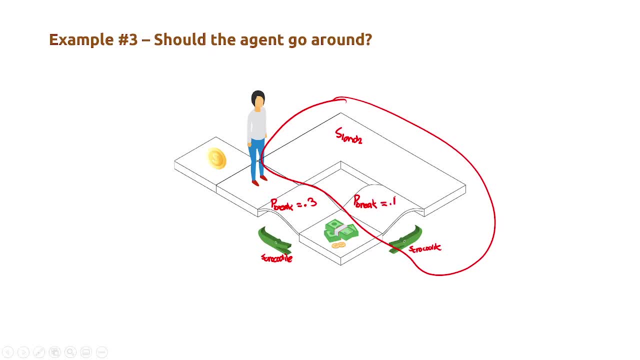 breaking, breaking of 0.1 of 0.1 of 0.1, so so, so this means that this bridge okay the second. this means that this bridge okay the second. this means that this bridge okay the second, the new bridge is. the new bridge is: 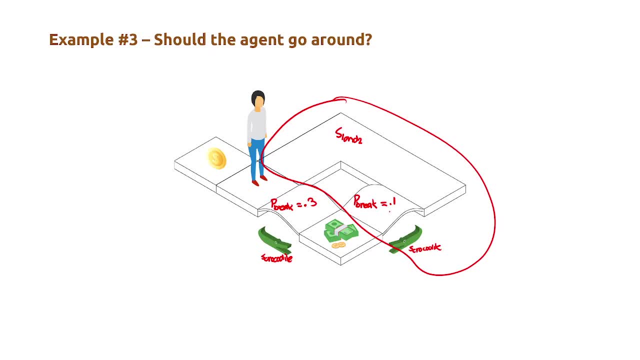 the new bridge is sturdier, sturdier, sturdier is sturdier, or more reliable than the is sturdier or more reliable than the is sturdier, or more reliable than the older bridge. so should our agent take the? so should our agent take the. 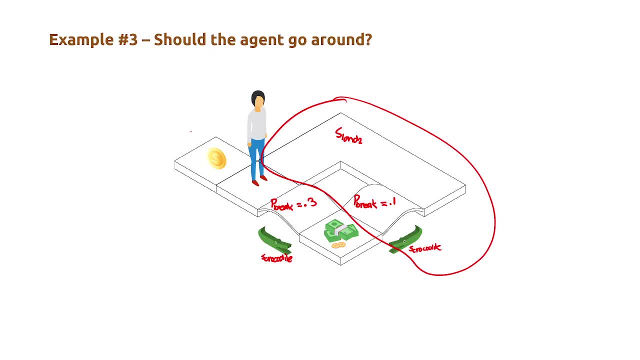 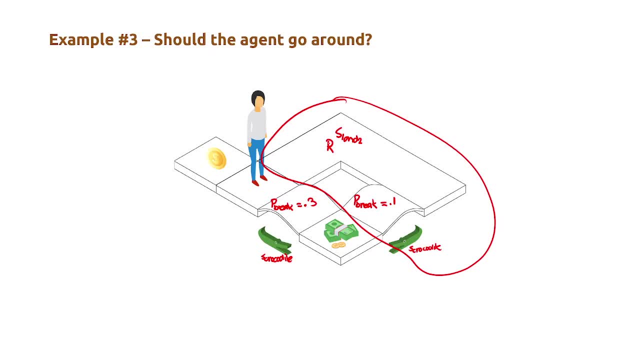 take note that the reward, take note that the reward when you, when the agent goes in this, when you when the agent goes in this, when you when the agent goes in this, or when the agent goes around, or when the agent goes around, or when the agent goes around, is negative 10 okay. 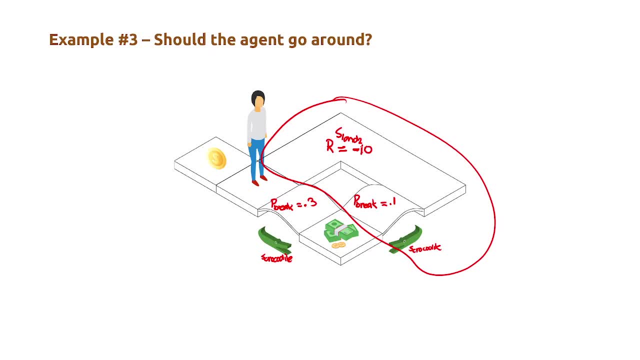 is negative 10, okay. is negative 10, okay. so we're also going to take that into. so we're also going to take that into. so we're also going to take that into account. account, account. so that again, the reward of. so that again, the reward of. 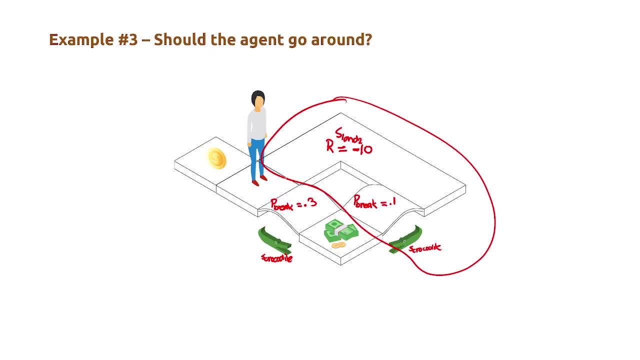 so that again, the reward of going around, going around, going around to this state, to this state, to this state, is negative 10. is negative, 10. is negative 10.. so again, we can represent this as the mark. so again we can represent this as the mark. 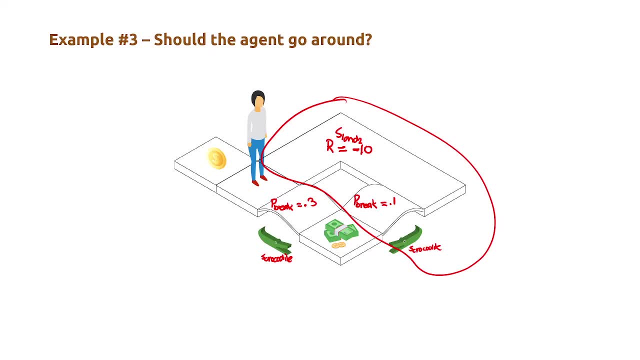 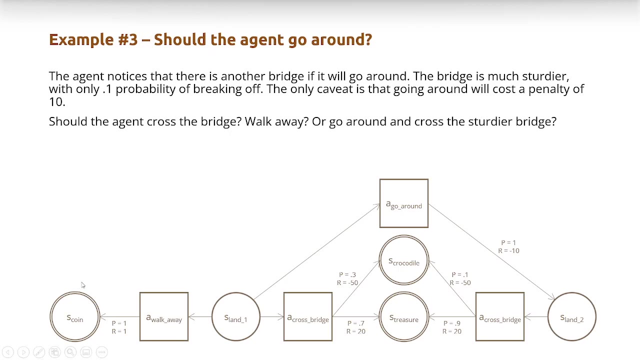 so, again, we can represent this as the mark of, of, of decision process. so we can represent this as the mark of. so we can represent this as the mark of, so we can represent this as the mark of decision process. so i just moved, so i just moved. 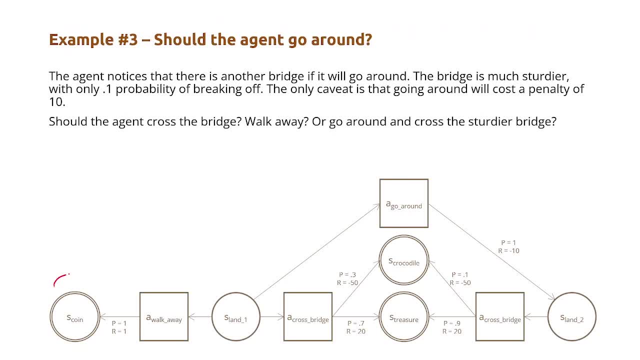 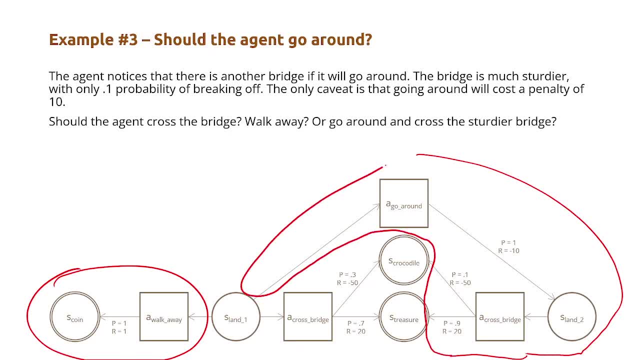 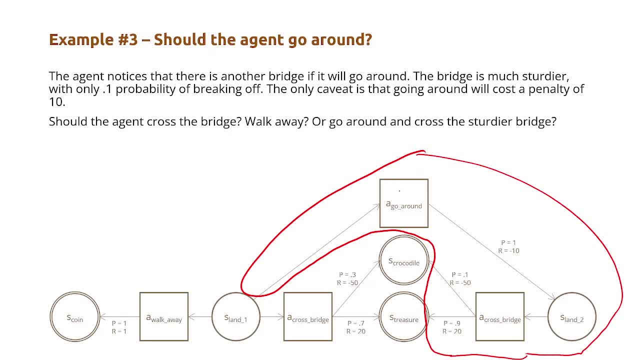 just extends, uh, the older, just extends, uh, the older mdp that we have created. i added the go mdp that we have created. i added the go mdp that we have created. i added the go around action, around action, around action. we go around action which transitions to 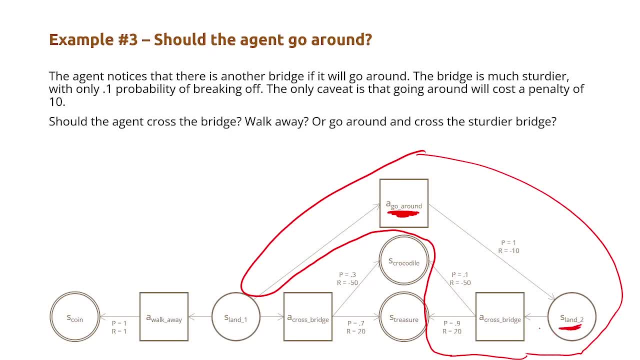 we go around action which transitions to. we go around action which transitions to: s land 2. s land 2. s land 2.. then, when you are in s land 2, you only. then when you are in s land 2, you only. 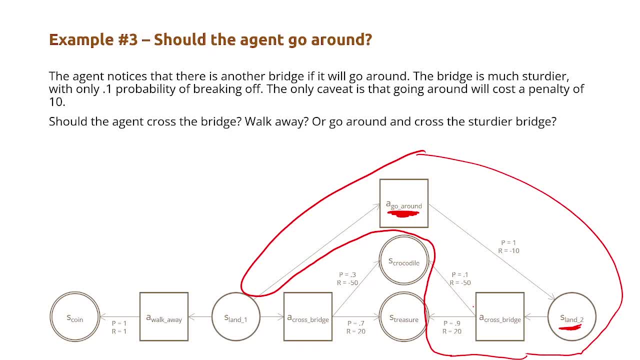 then, when you are in s land 2, you only have one action which is which is to have one action, which is which is to have one action which is which is to cross the bridge, cross the bridge, cross the bridge, crocodile. and then there is a point. 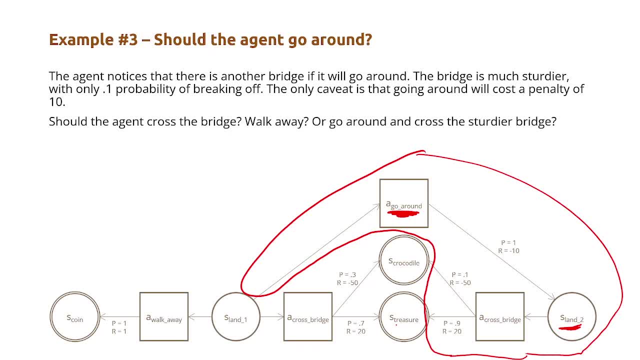 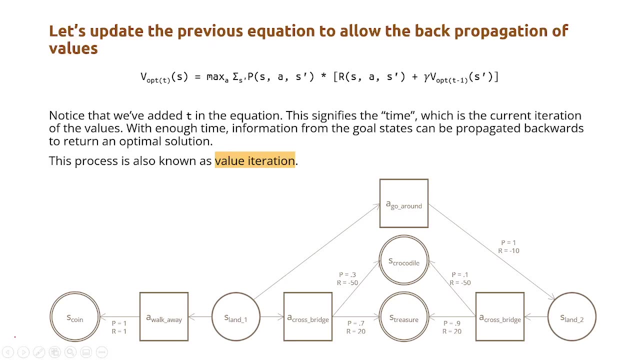 crocodile, and then there is a point crocodile, and then there is a point: time, probability of time, probability of time, probability of actually arriving to the treasure on that side. so again, we update our, so again we update our, so again we update our previous equation to allow the back. 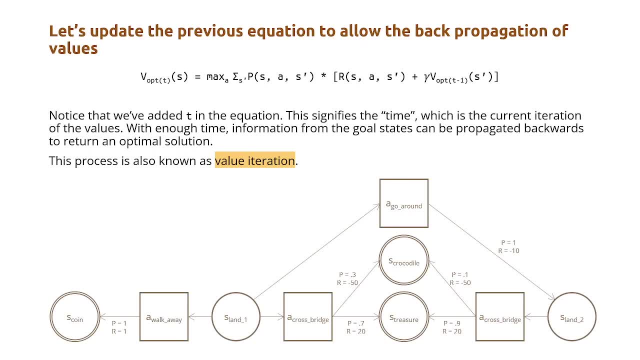 previous equation to allow the back. previous equation to allow the back. propagation of values. propagation of values. propagation of values. so notice that we have added. so notice that we have added. so notice that we have added t. okay, we have added t. t. okay, we have added t. okay, we have added t. 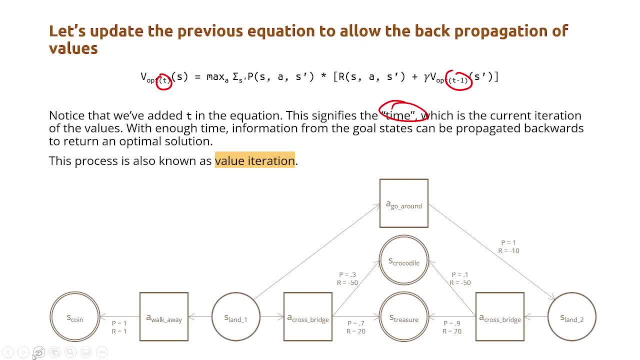 t. okay, we have added t. okay, we have added t. so the t signifies time. e signifies time, which is the current. e signifies time which is the current. e signifies time, which is the current iteration of the values, iteration of the values. iteration of the values with enough time. information from the 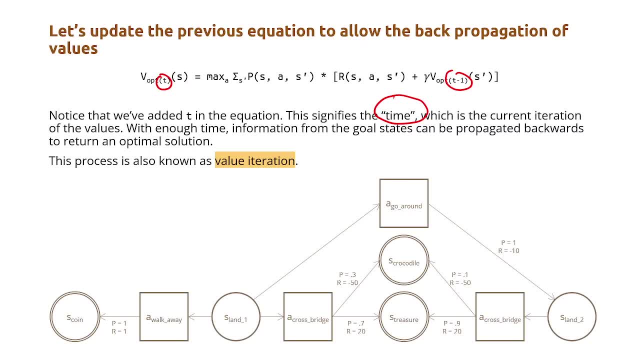 with enough time, information from the- with enough time, information from the goal states can be propagated backwards. goal states can be propagated backwards. goal states can be propagated backwards to return an optimal solution. to return an optimal solution, to return an optimal solution. this process is also known as value. 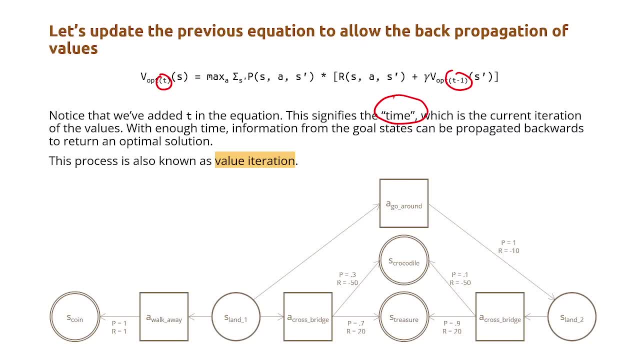 this process is also known as value. this process is also known as value iteration, iteration, iteration. so basically the algorithm of value. so basically the algorithm of value. so basically the algorithm of value. iteration is just to repeat and repeat. iteration is just to repeat and repeat. iteration is just to repeat and repeat the process of calculating the values. 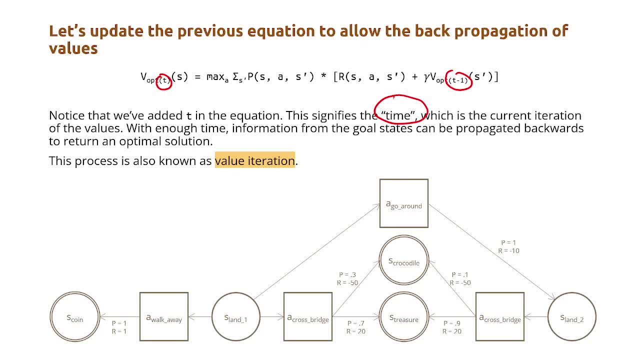 the process of calculating the values. the process of calculating the values until until. until, okay, until the values do not change. okay, until the values do not change. okay, until the values do not change anymore. so that's what we call the anymore. so that's what we call the. 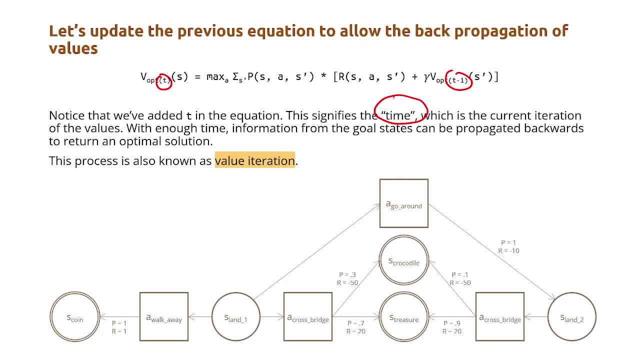 anymore. so that's what we call the convergence, convergence. convergence which i will show, in which i will show, in which i will show in a while. okay, so, for the first, a while. okay, so, for the first, a while. okay, so for the first iteration, iteration, iteration, okay for the first iteration, or at t is: 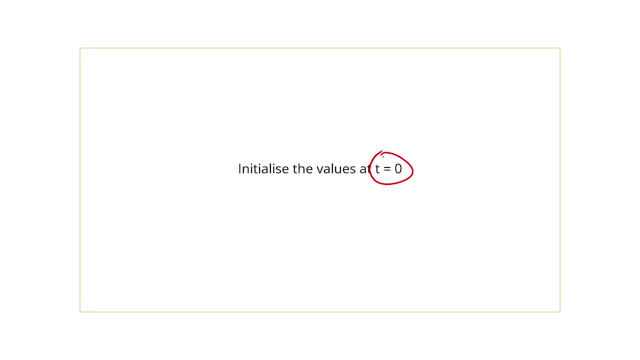 okay for the first iteration. or at t is okay for the first iteration. or at t is equal to zero. equal to zero, equal to zero. at t is equal to zero. we initialize the. at t is equal to zero. we initialize the. at t is equal to zero. we initialize the values to zero. 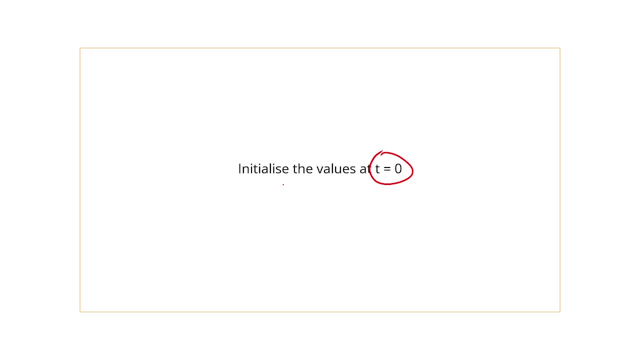 values to zero, values to zero, so what do we? what do we mean by so? what do we? what do we mean by? so what do we? what do we mean by initializing the values to zero? so, initializing the values to zero, so, initializing the values to zero. so remember that we have, uh, one, two, three. 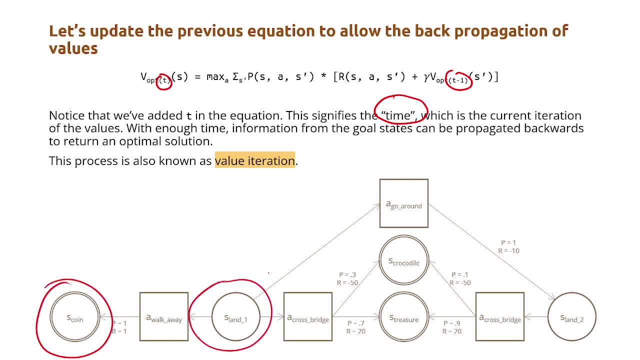 remember that we have uh one, two, three. remember that we have uh one, two, three, four. five states right. four. five states right four. five states right: one state, second state, third state, one state, second state, third state, one state, second state, third state, fourth state and fifth state. 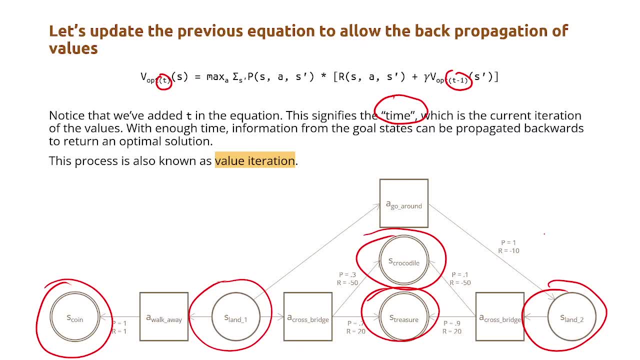 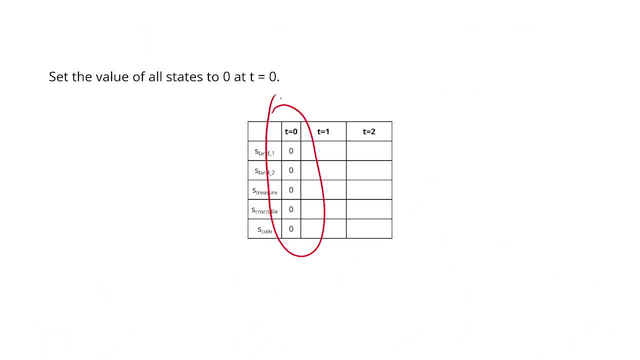 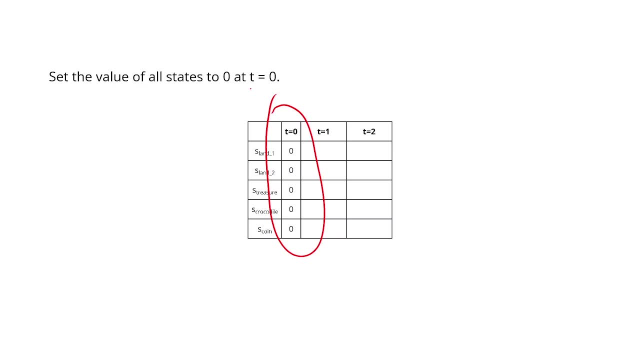 it's one right here, so set all the. it's one right here, so set all the. it's one right here, so set all the values of all states to zero at values of all states to zero. at values of all states to zero. at t is equal to zero. 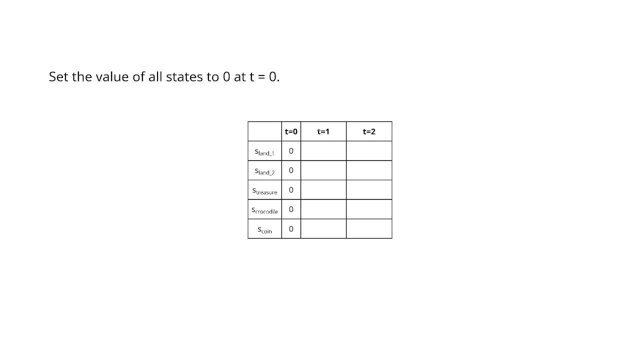 so after that, after we have calculated, so after that, after we have calculated, so after that, after we have calculated, t is equal to zero, t is equal to zero, t is equal to zero. we will now calculate t is equal to one. yeah, calculate the values at t is equal. 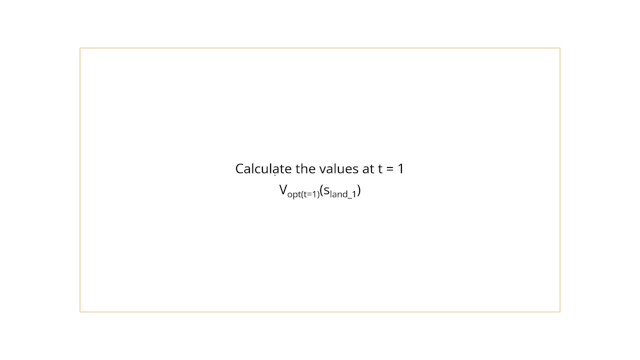 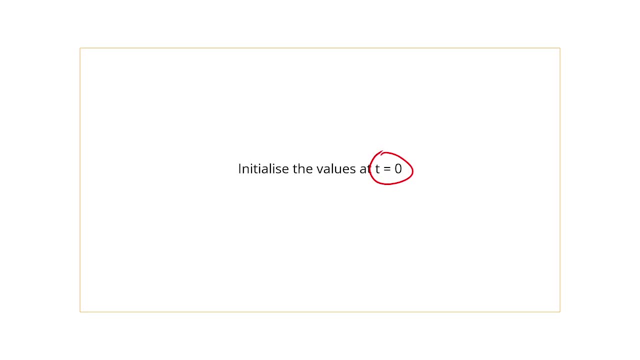 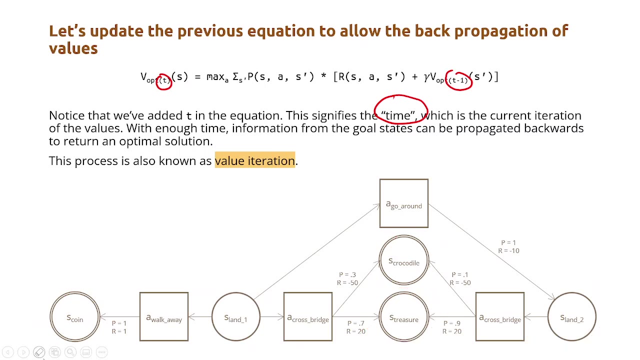 um, by the way, by the way, by the way. um, by the way, by the way, by the way, um, by the way, by the way, by the way. so, okay, um, okay, um, okay, um. the the goals it's, or the states with the the goals it's, or the states with. 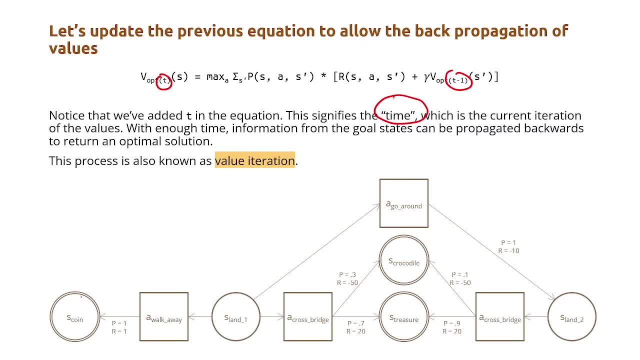 the, the goals it's, or the states with two circles, two circles, two circles. their values will be zero all throughout the. their values will be zero all throughout the. their values will be zero all throughout the time, time, time. okay. however, the value of the states, of the? 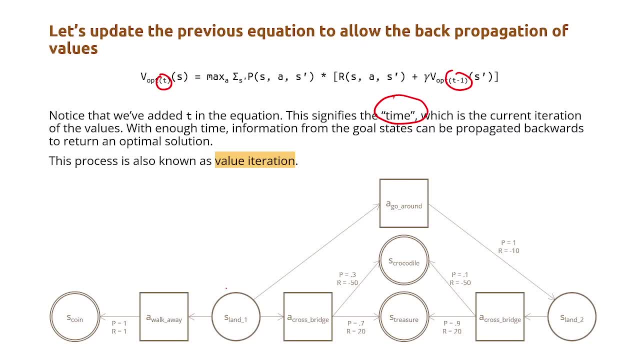 okay. however, the value of the states of the? okay. however, the value of the states, of the states that are not final states, states that are not final states, states that are not final states, will change depending on. will change depending on. will change depending on how the values are being propagated. okay, 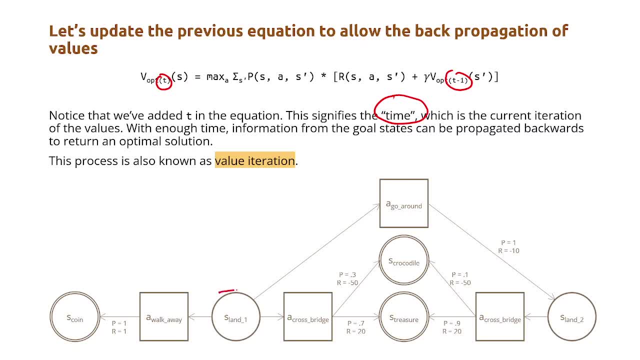 how the values are being propagated, okay, how the values are being propagated, okay, so, basically, so, basically, so, basically, the values that we're just going to, the values that we're just going to, the values that we're just going to calculate: is this calculate? is this calculate? is this slan1 and slan2? so again, we will. 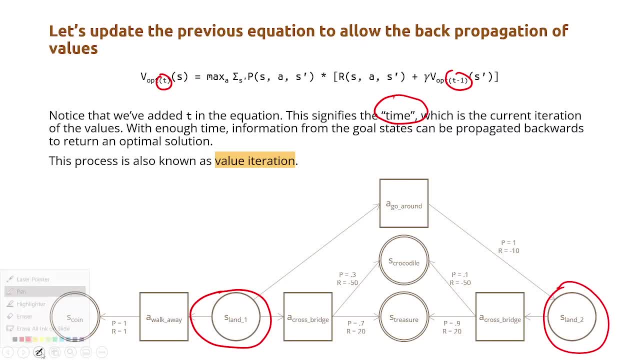 slan1 and slan2. so again we will: slan1 and slan2. so again we will calculate the values of slan1 and slan2. calculate the values of slan1 and slan2. calculate the values of slan1 and slan2 only. 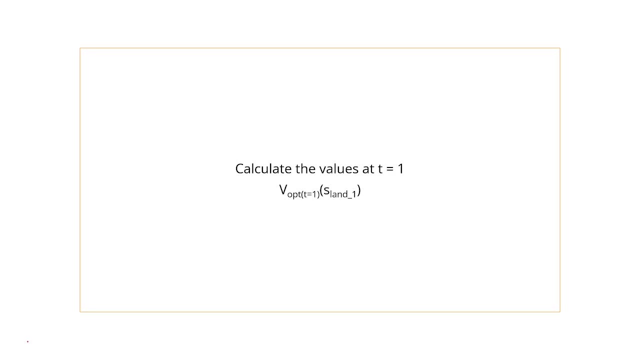 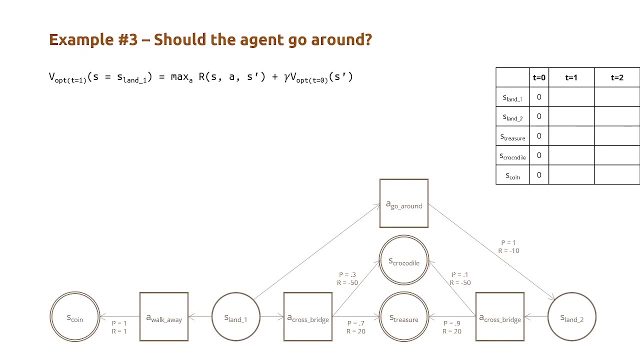 right. so again calculate the values at t right. so again calculate the values at t right. so again calculate the values at: t is equal to one, is equal to one, is equal to one of slan1. so yes, um, um, um. okay, so this equation is stacking. 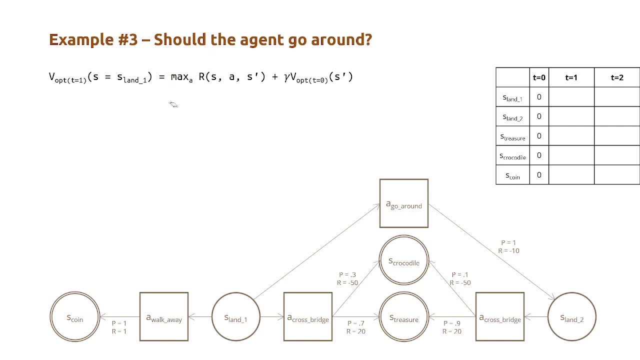 okay, so this equation is stacking. okay, so this equation is stacking. remember, remember, remember, remember. one crossing the bridge and transitioning, one crossing the bridge and transitioning, one crossing the bridge and transitioning to crocodile, to crocodile, to crocodile. so probability is 0.3. so probability is 0.3. 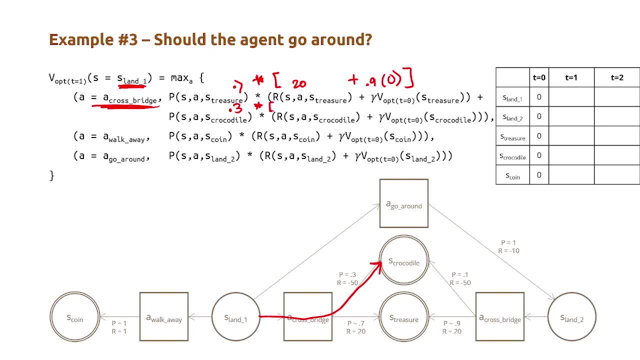 so probability is 0.3, three times, three times, three times the reward of negative, 50 plus plus plus 0.9, which is our 0.9, which is our 0.9, which is our gamma times, gamma times, gamma times v opt. optimal value of. 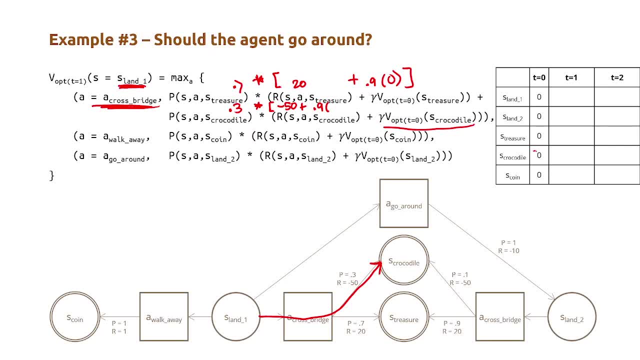 v opt. optimal value of v opt. optimal value of crocodile- crocodile crocodile. as for hudal, at time is equal to zero. it is as for hudal, at time is equal to zero. it is. as for hudal, at time is equal to zero. it is equal to zero. 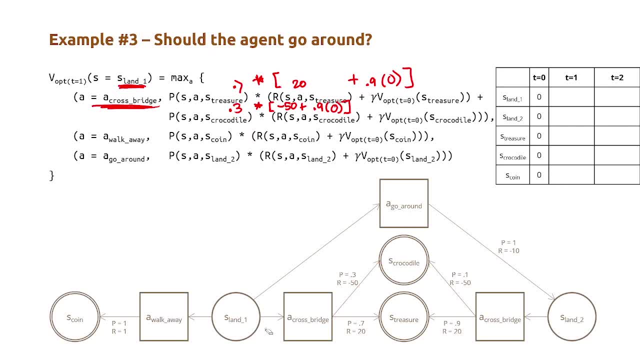 next: uh-huh, okay, uh-huh, okay, uh-huh, okay. next, we calculate the value of this path. next, we calculate the value of this path. next, we calculate the value of this path. so what's the probability? the so what's the probability? the so what's the probability? the probability is one. 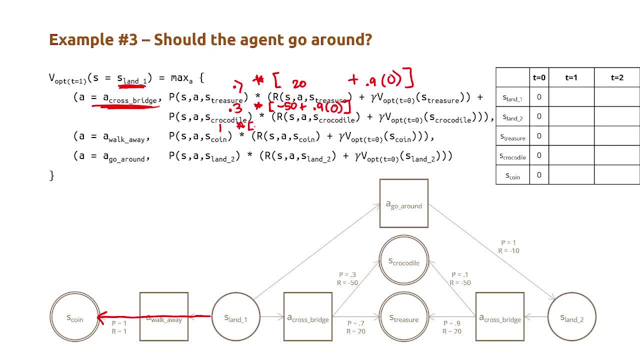 probability is one probability is one multiplied by the reward of one, multiplied by the reward of one, multiplied by the reward of one plus gamma of 0.9, plus gamma of 0.9, plus gamma of 0.9 times the value. times the value. 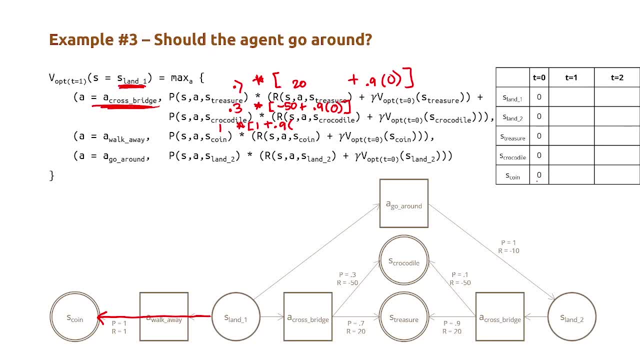 times the value of the value of s coin at time is equal to of the value of s coin at time is equal to of the value of s coin at time is equal to zero, which is basically zero, which is basically zero, which is basically zero. lastly, we calculate: 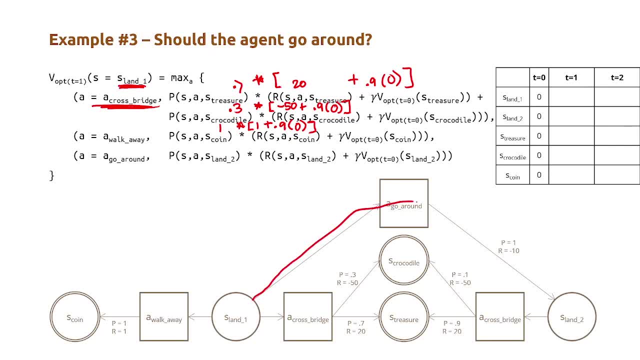 lastly, we calculate. lastly, we calculate: um the path, um the path, um the path, the value of this path, the value of this path, the value of this path. so, given the action go around, what is the so, given the action go around, what is the so, given the action go around, what is the probability? 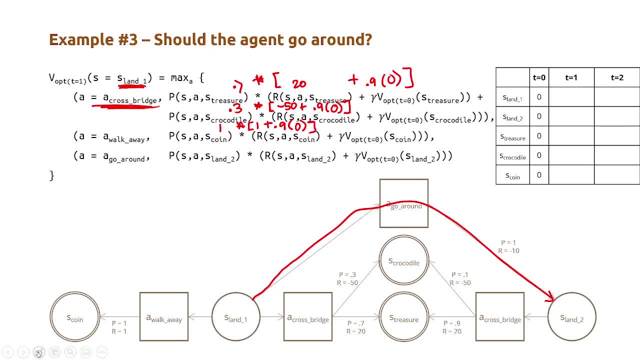 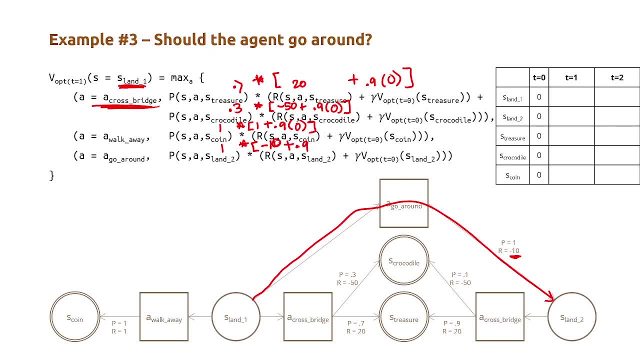 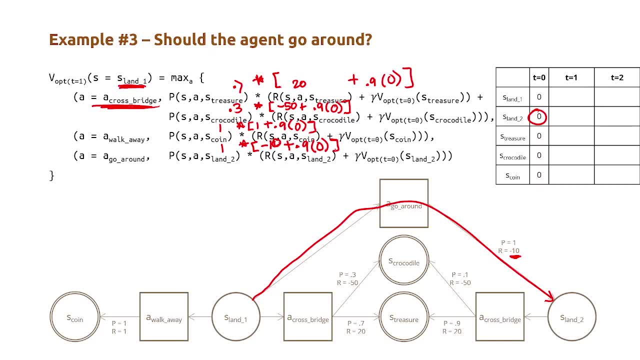 time is equal to zero, so this is zero. okay, so it looks. i think, uh what i've? okay, so it looks. i think, uh what i've okay, so it looks. i think, uh, what i've written is correct, so let's proceed to. written is correct, so let's proceed to. 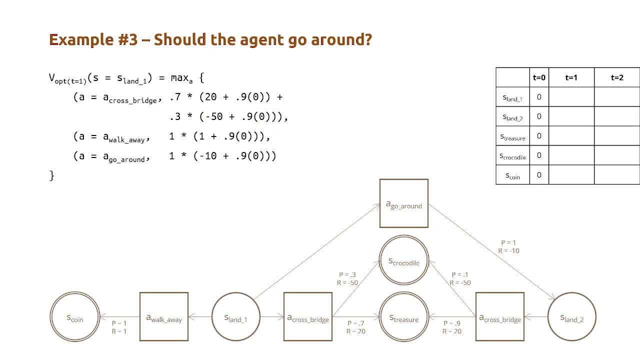 written is correct, so let's proceed to the next slide. the next slide, the next slide. okay, okay, okay. next slide, next slide, next slide. oh yeah, it's basically just the same. oh yeah, it's basically just the same. oh yeah, it's basically just the same from what i've written in the previous. 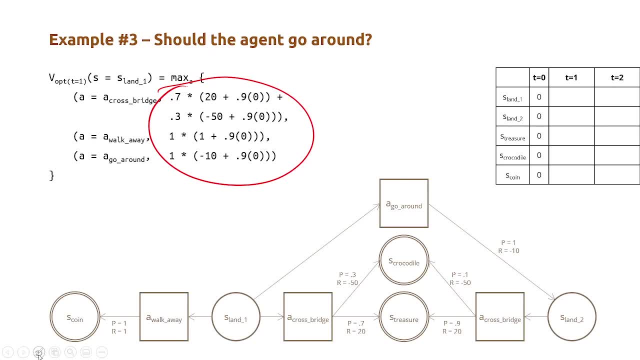 from what i've written in the previous, from what i've written in the previous: slide, slide, slide distance. so remember again, so remember again, so remember again, remember that we add these two things, remember that we add these two things, remember that we add these two things. okay, we add these two things because 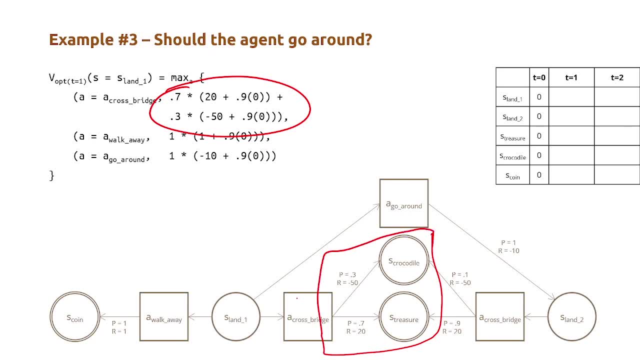 okay, we add these two things because. okay, we add these two things because they are in the same action. they are in the same action. they are in the same action. we just want the. we just want one value. we just want the. we just want one value. we just want the. we just want one value for cross bridge. 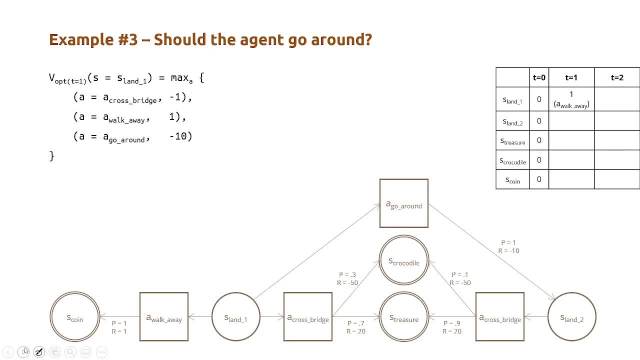 so, after we evaluate these equations, we so, after we evaluate these equations, we so, after we evaluate these equations, we are given to these values are given to these values are given to these values. so which one is the maximum negative one? so which one is the maximum negative one? 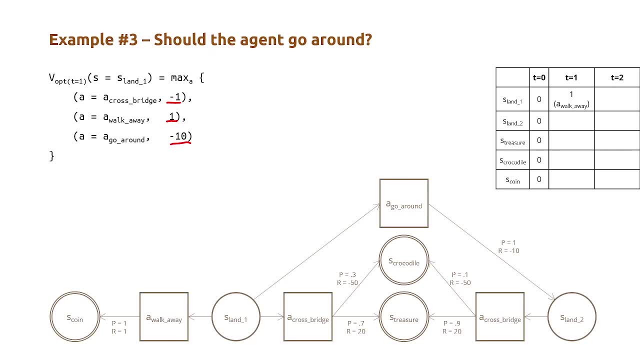 so which one is the maximum? negative one one or negative ten, one or negative ten, one or negative ten. so obviously the maximum value is one, so obviously the maximum value is one. so obviously the maximum value is one and the and the and the. the action is walk away right. so in the 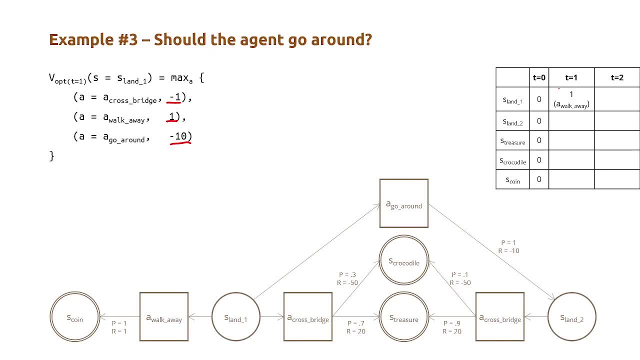 the action is walk away right. so in the, the action is walk away right. so in the right side, right side, right side of our uh, in the right side in our table of our uh, in the right side in our table of our uh, in the right side in our table, we write one and we also write walk away. 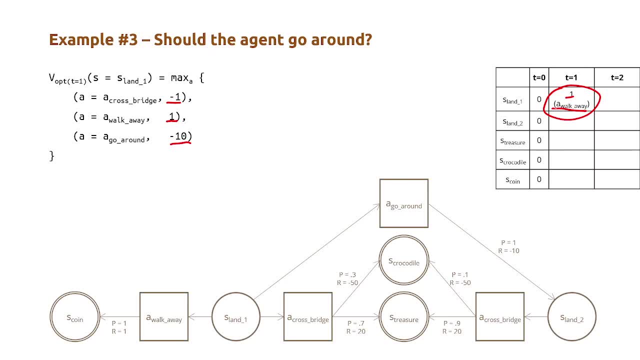 we write one and we also write walk away. we write one and we also write walk away. so this tells us that walk away. so this tells us that walk away. so this tells us that walk away provided the highest value for. so this tells us that walk away provided the highest value for. 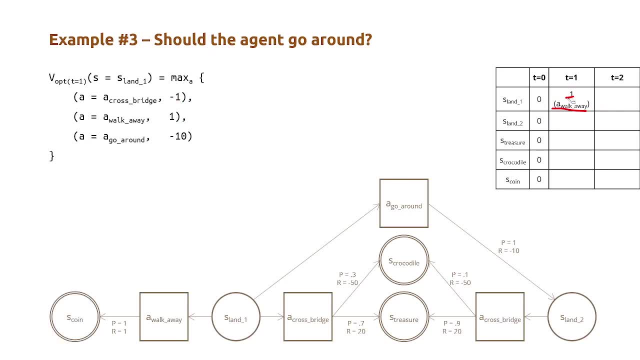 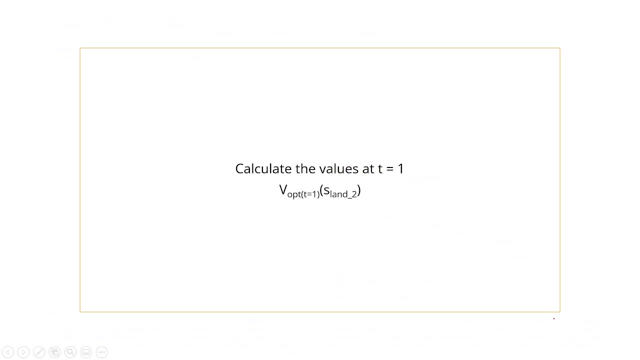 so this tells us that walk away provided the highest value for next. we calculate the value of next. we calculate the value of next. we calculate the value of s92. calculate the value of s92 at t is equal. calculate the value of s92 at t is equal. 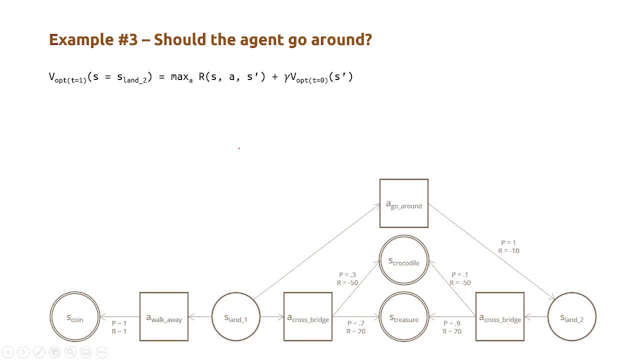 calculate the value of s92 at t is equal to one. so yeah, another drill. so yeah, another drill. so yeah, another drill. so yeah, we have two paths first we have. so yeah, we have two paths first we have. so yeah, we have two paths first. we have this path. 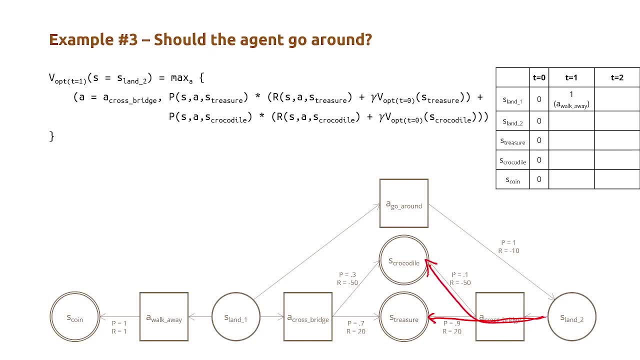 this path, this path, then we have this path, then we have this path, then we have this path. right, right, right, so, so, so, so, so, uh, okay, so what's the probability of? uh, okay, so what's the probability of uh, okay, so what's the probability of going to the treasure when you're s in? 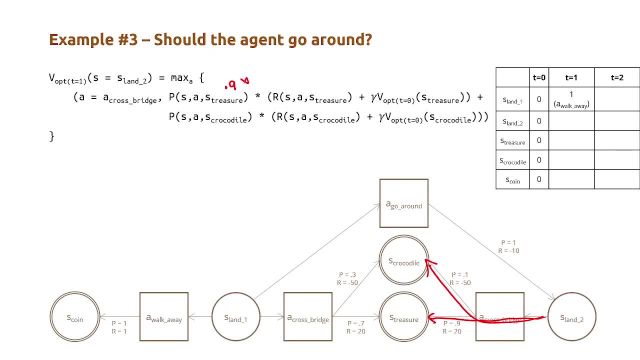 going to the treasure when you're s in going to the treasure when you're s in s92, it is 0.9, s92, it is 0.9, s92, it is 0.9. nine times the reward of is 20.. 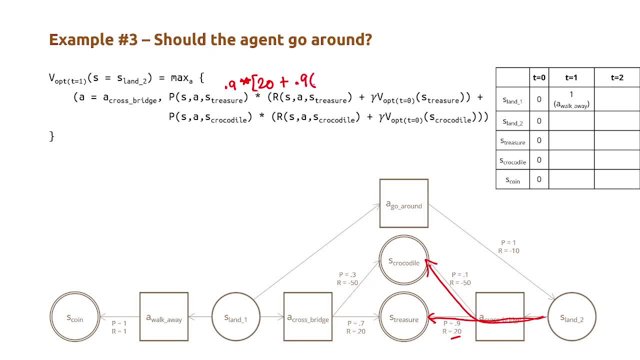 nine times the reward of is 20.. nine times the reward of is 20.. plus gamma of 0.9 plus gamma of 0.9. plus gamma of 0.9, times times times, the opt of s treasure at time is equal. 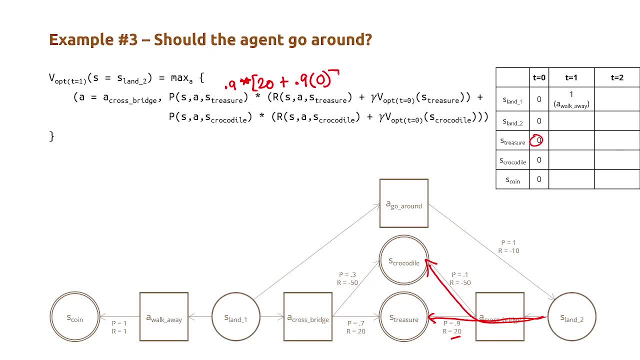 the opt of s treasure at time is equal, the opt of s treasure at time is equal to zero, to zero, to zero is zero. then then then, below we have, below, we have, below we have, yeah, crocodile the crocodile path. so, yeah, crocodile, the crocodile path, so 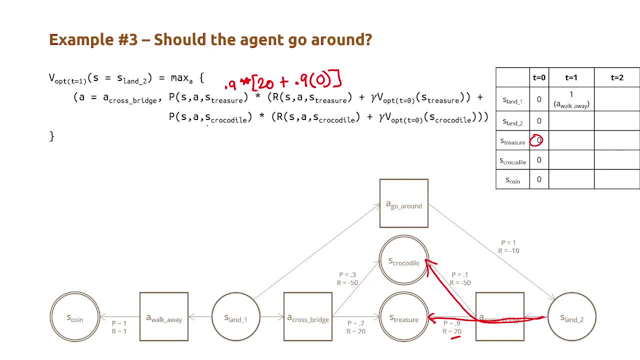 yeah, crocodile, the crocodile path. so what's the probability of going to the? what's the probability of going to the? what's the probability of going to the crocodile when crossing the bridge at crocodile when crossing the bridge at crocodile. when crossing the bridge at s2? it is 0.1. 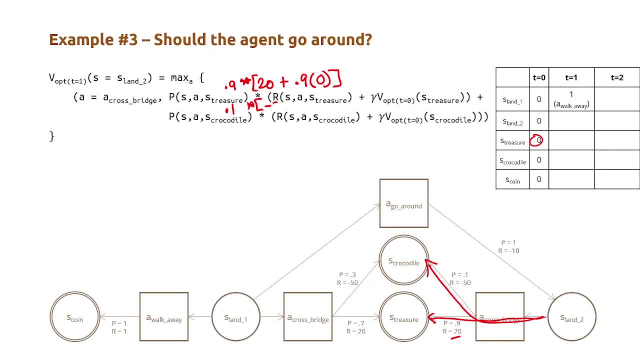 s2. it is 0.1 s2. it is 0.1 times times times the reward of negative: 50. um plus um plus um plus 0.9, 0.9, 0.9 times times times. Insert 0.9 timescom. 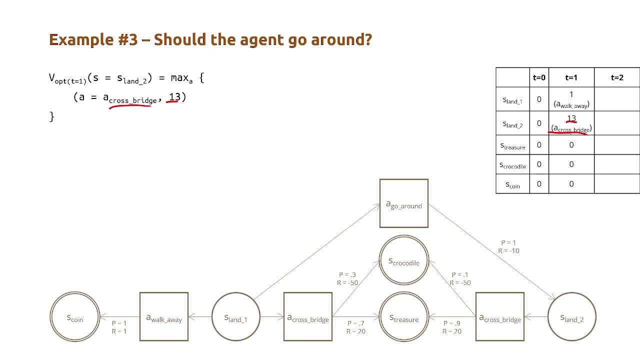 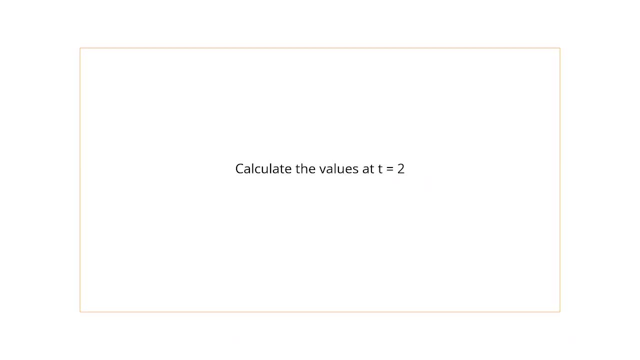 0.9 timescom. 0.9 X 0. 0.9 X 0. Next. Yeah, so we just set the values of S-threshold, S-coordinate and S. going to zero at t is equal to one, because we are final states. 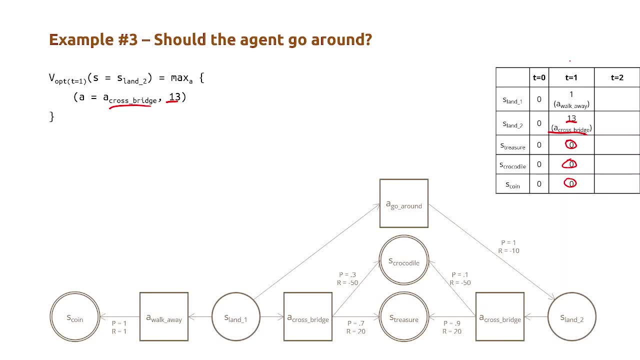 Calculate the values at t is equal to two. So okay, so we have finished calculating: the values at t is equal to one. Next we have to calculate: the values at t is equal to two. Right, So we just repeat the process. 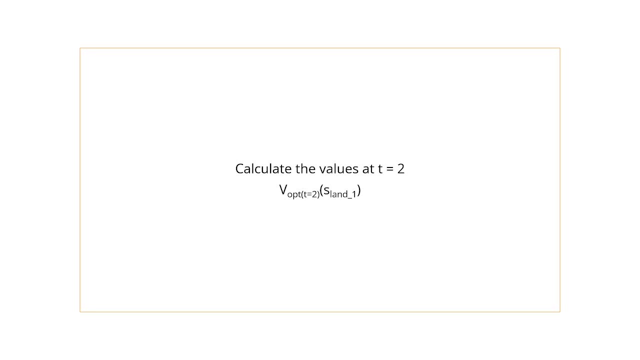 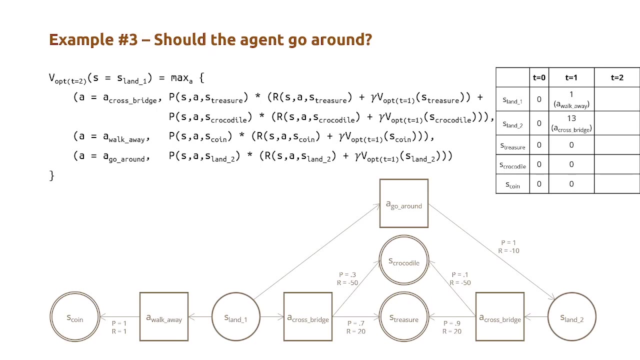 Calculate again the optimal value of the S-land. one at t is equal to two. Okay, Next. So what's the probability of going to the treasure when crossing the bridge? It is 0.7.. Reward is 20.. Gam of 0.9.. 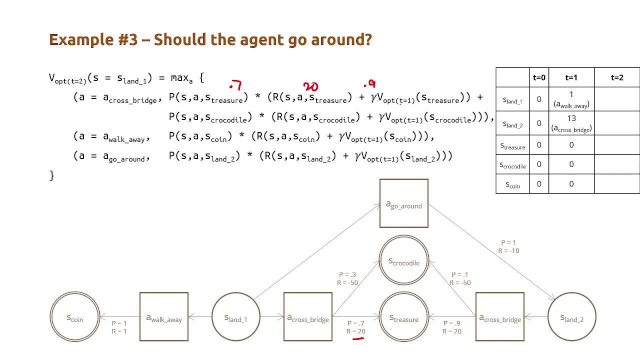 Okay, So notice that. Okay, wait, So take a look here. take a look here, So notice that t is equal, is now equal to two right, And then here t is equal to one. So this is where the back propagation. 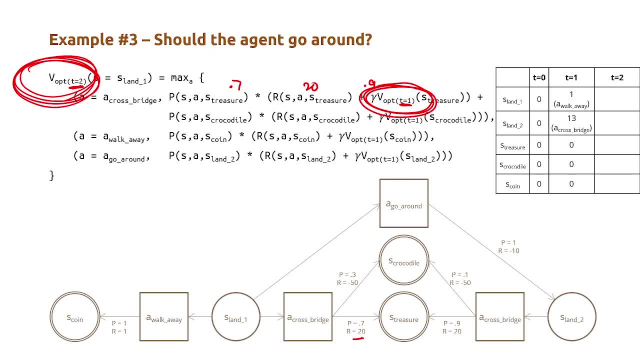 where you can like see the back propagation. So we basically look back to the previous value of the treasure, Okay, And then we can see that it's not in the state. So what's the optimal value of treasure at t is equal to one. 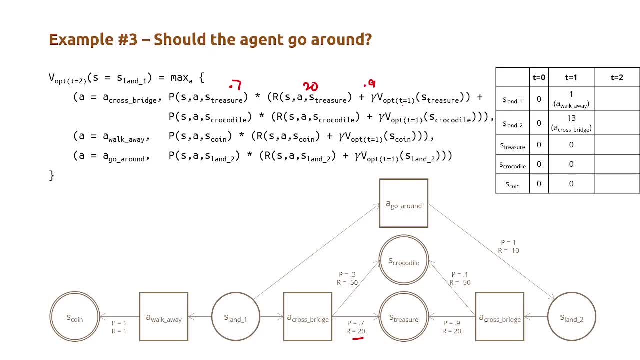 It is zero, It's just zero, Easy. Next, what is the probability of going to the codile when crossing the bridge at S-land? one, It is 0.3.. Reward is negative: 15.. And then the next one is the probability of going to the codile. 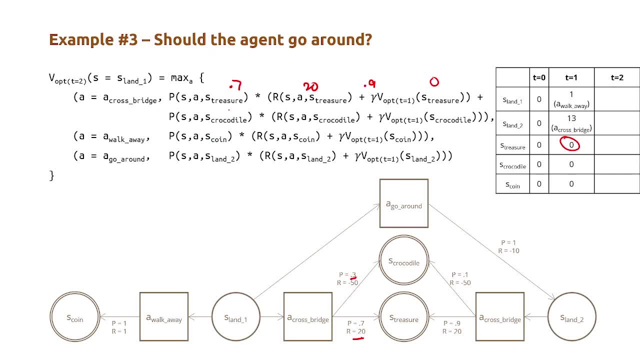 when crossing the bridge at S-land one. It is 0.3.. Reward is negative: 15.. Okay, It is 0.3 plus 0.9 of gamma multiplied by the value of S-crocodile at t is equal to one, which is zero. 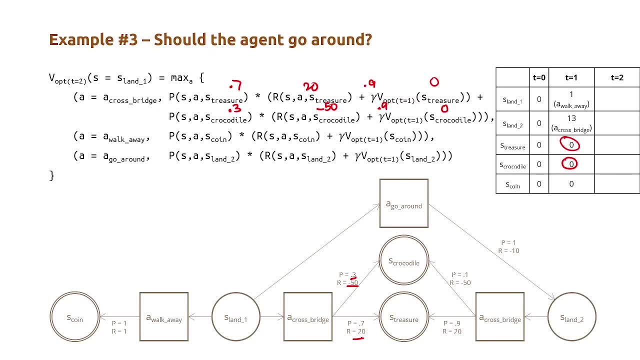 Next we calculate the value when walking away. So what is the probability of going to the coin when walking away? It is one. The reward is also one. Okay, Reward is one Gamma 0.9.. Optimal value of S-coin at t is equal to one is zero. 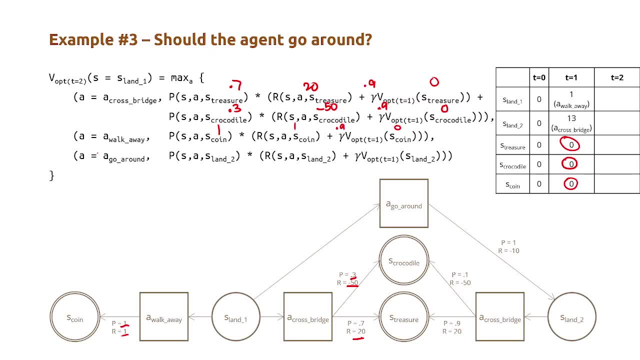 Okay. Next, if we go around, what's the probability of landing or arriving at S-land two when going around? It is one, Okay, The reward is negative 10.. Gamma is 0.9.. And okay, so this is where things get a little bit exciting. 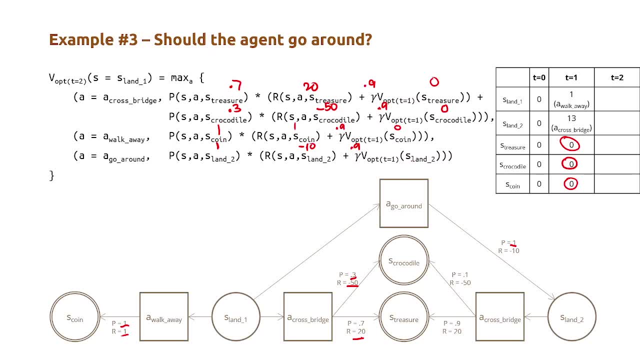 So so vopt Okay. Optimal value of S-Land: two at t is equal to one, is not zero, It is 13. So, right, 13. Okay. So now look Okay. so if we go, let me just fix the equations real quick. 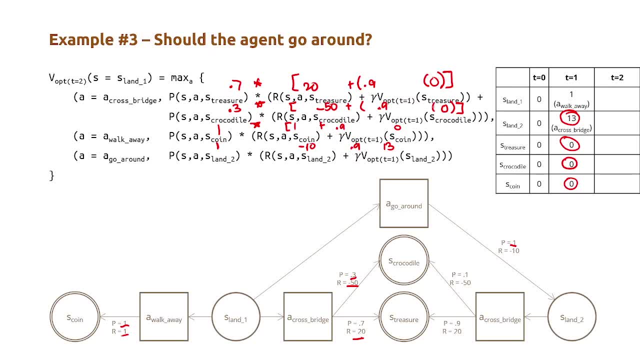 Okay, so that's how the equations will look like. So if we go to the next slide, it will just be the same, Okay, yeah, so it's just the same, right? Okay, so it's the same. So if we evaluate the values, we get this result. 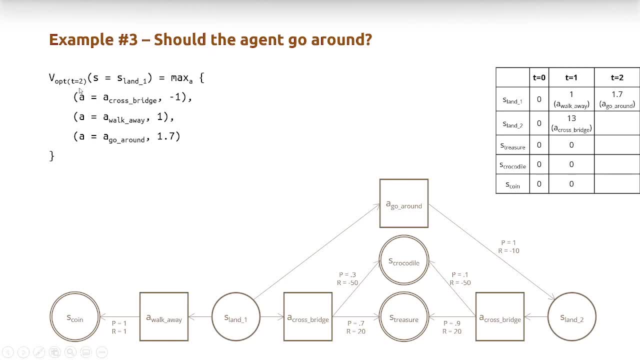 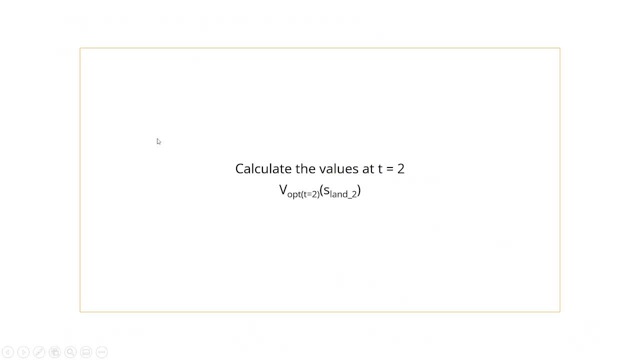 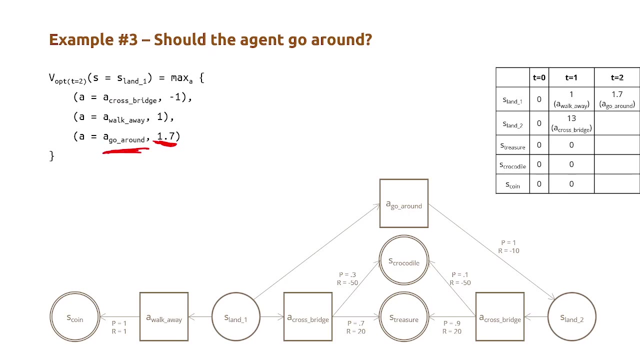 So now the value of s than 1 at t is equal to 2 will be the maximum value of this, which is 1.7.. 1.7.. And then the action is 1.. So now we update: t is equal to 2 of s than 1,. value of s than 1 at t is equal to 2, 1.7.. 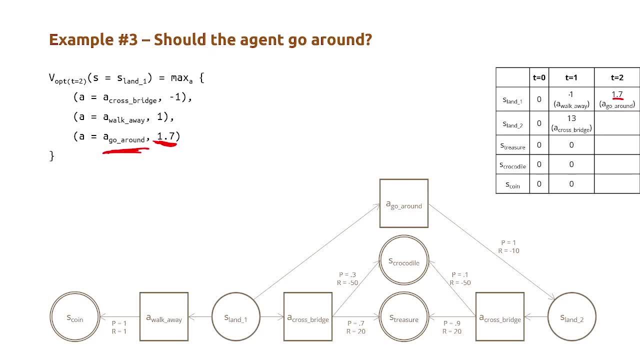 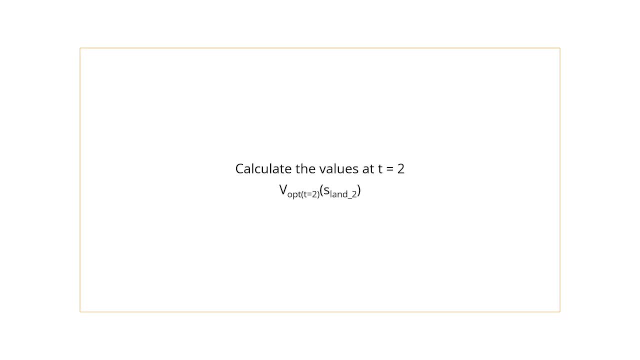 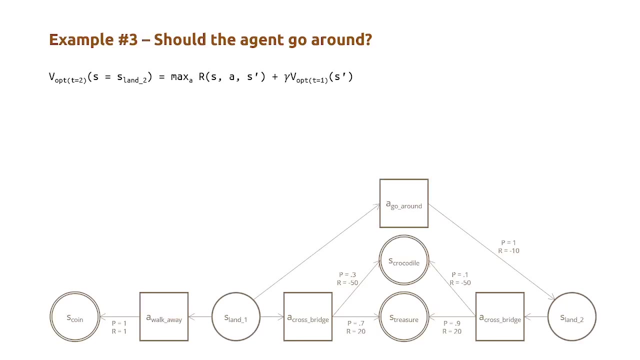 And then the action now is updated from walk away, it will not change. to go around, Okay. next We calculate the value of s than 2 at t is equal to 2.. Okay, so, yeah, What's the probability of? 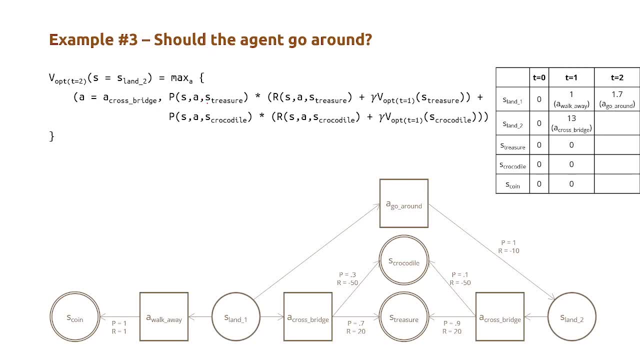 Arriving at. Arriving at Arriving at The state treasure when crossing the bridge, it is 0.9.. 0.9 times the reward Reward is 20.. 20 plus gamma of 0.9 times v opt at t1 of treasure is 0.. 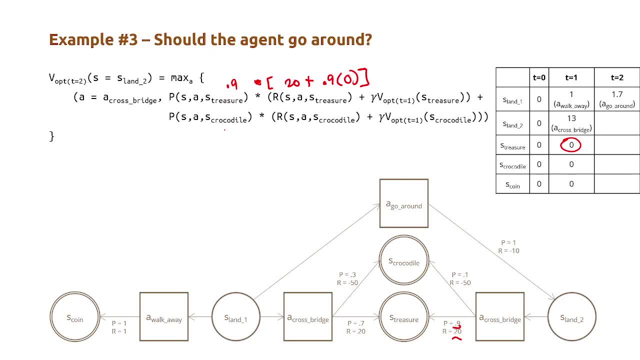 Then below we have probability We have probability of, And then below we have probability of Arriving at the crocodile when crossing the bridge. it's 0.1 times reward of negative 50 plus 0.9 times optimal value of s crocodile at t is equal to 1.. 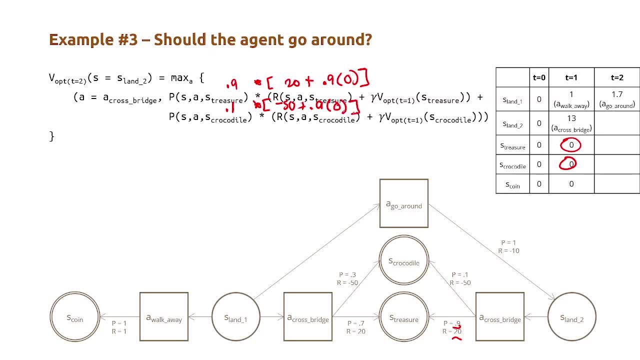 Arriving at the crocodile when crossing the bridge. it's 0.1 times reward of negative 50 plus 0.9 times optimal value of s crocodile at t is equal to 1. Which is 0.. Which is 0.. 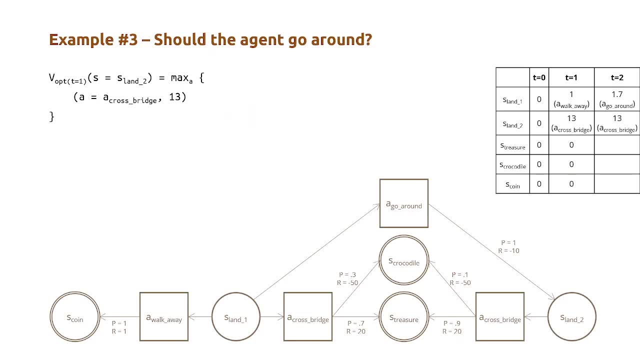 Result in this value, Crossing the bridge is equal to 30.. Okay, So the maximum value is 13 and the action is cross the bridge. So notice that. s then 2. did that change? Okay, It's still the same: 13 and cross the bridge. 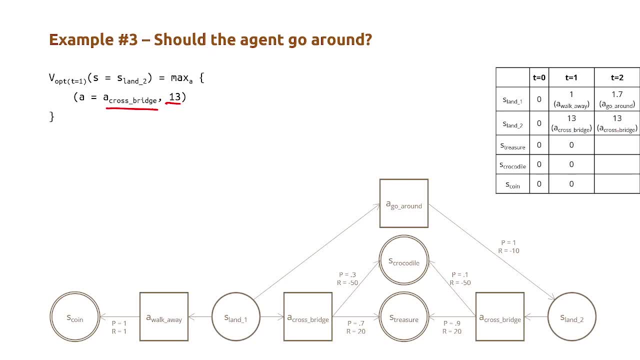 the bridge. also, we set the values of treasure, crocodile and coin to zero because again, they are dual states. okay, so we repeat the process again at: t is equal to three, okay, however, uh, i will not show it anymore, but basically, when we calculate the values again, 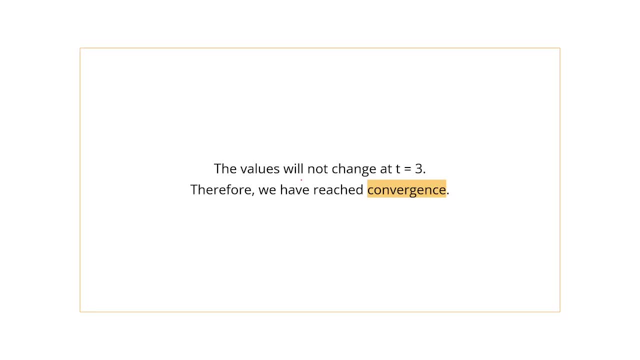 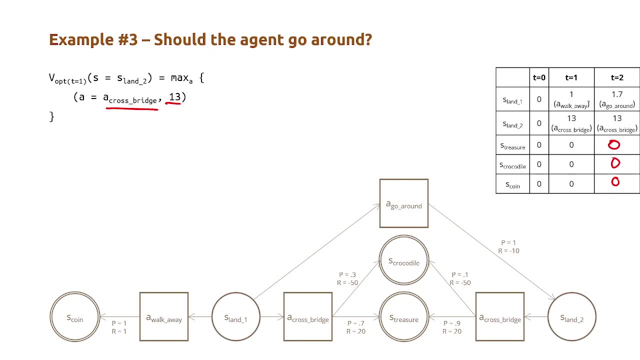 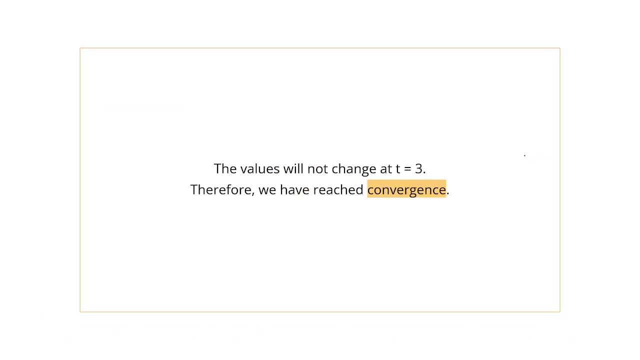 at t is equal to three. the values will not change anymore. so, basically, at t is equal to three. the value of sn1 is: it will be 1.7 with the action of going around. the value at s92 is also 13 when crossing the bridge. okay, at t is equal to three. therefore, because the values have not 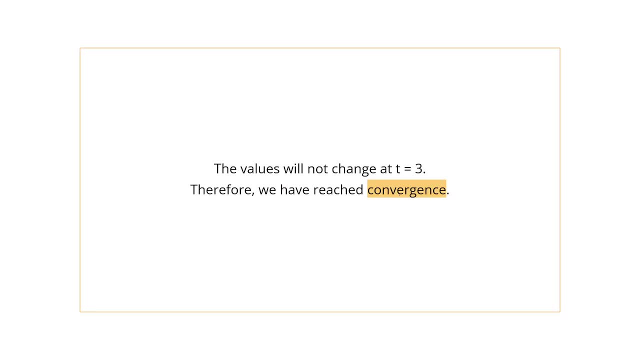 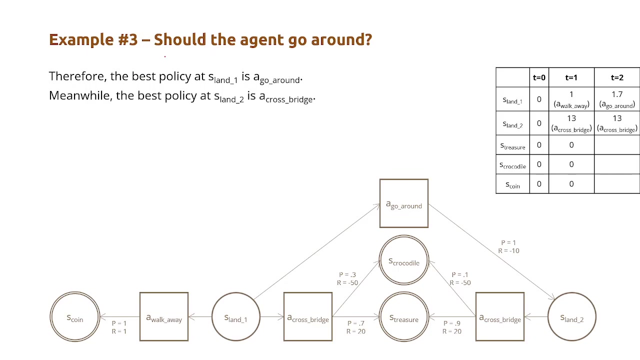 changed at. t is equal to three, we have reached convergence. so because we have reached convergence, we have found the solution of our um, we have found the solution to our mdp. so yeah, therefore, the best policy is at s land one is go around. the best policy at sn2 is cross the bridge, okay, so i hope that's clear. 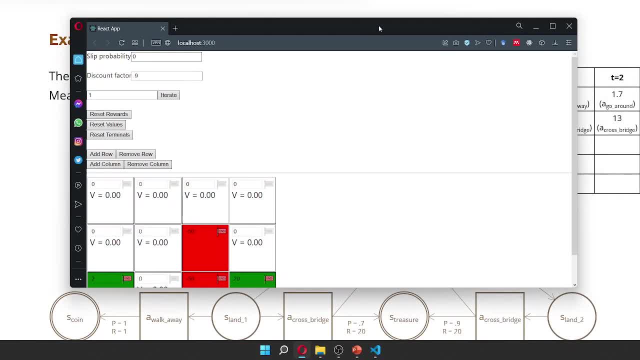 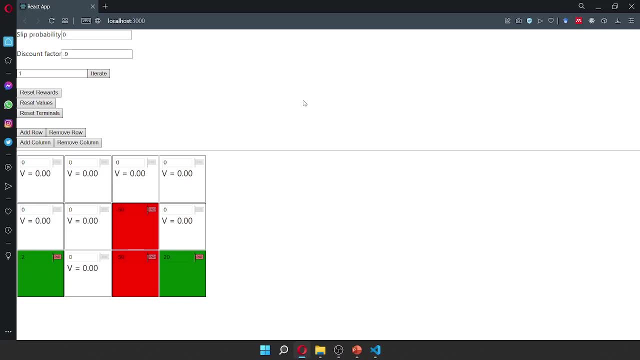 it's so clear. now let me show you something. so here i have. i made a simple web application, um, that represents the grid world and also value iteration, okay, so, yeah, as you all know, um, squares here below represent the states. okay, these squares represent the states um. 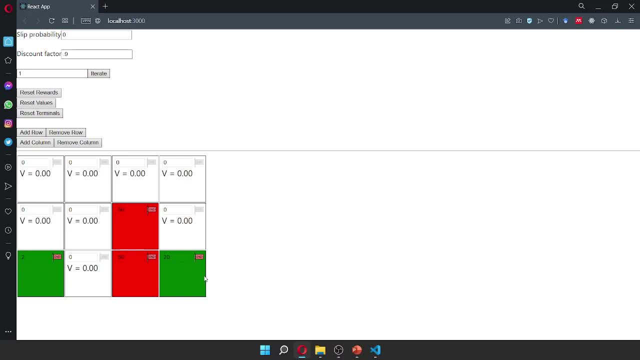 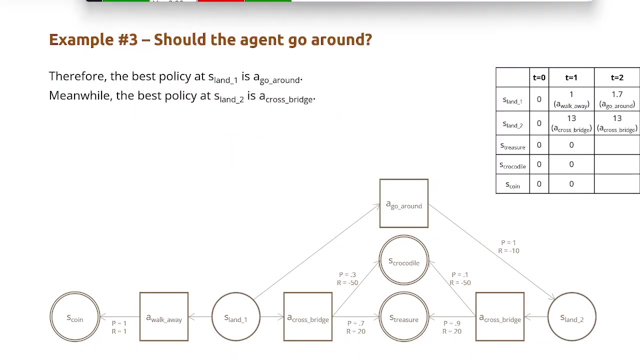 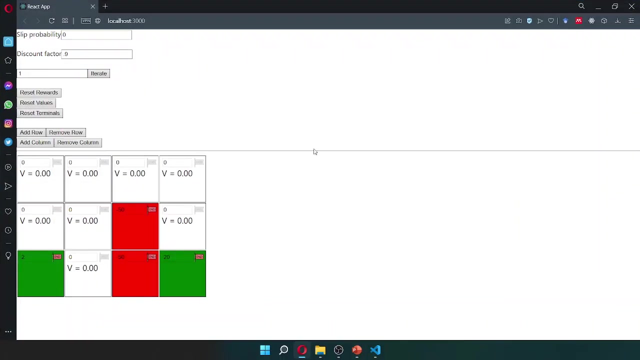 the green ones are positive rewards, the red ones are negative rewards. also, when you, when you arrive at these red and green states, you can see my mouse. let me just close the out. okay, there, it is okay. so again, uh, yeah, this is a grid world. each square represents the state. 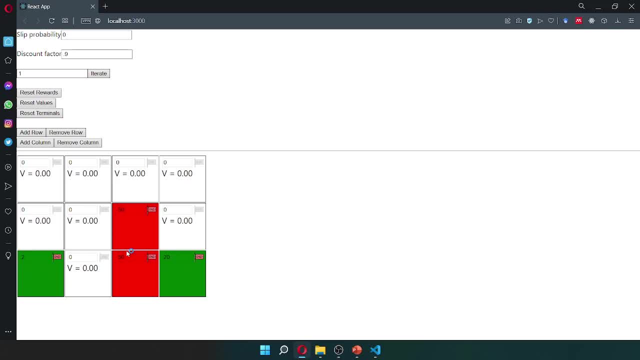 the green squares are positive rewards, the red squares are negative rewards, and if the agent arrives at at either red or greens squares, the game will end okay. so what we want to do, we want our agent to learn. we want our agent to learn basically all that: how to. 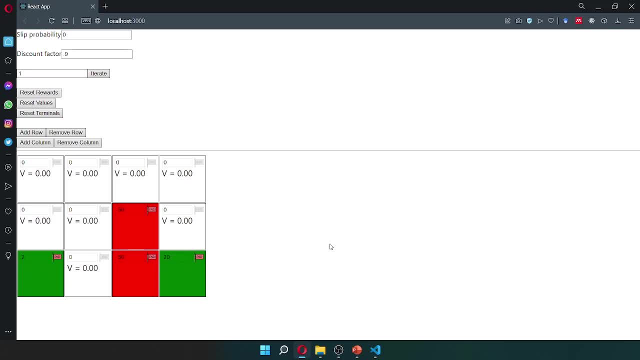 maximize the reward in the long run. okay, we want our agent to learn to maximize in the world long run. so let's just say that anyway, okay. so, yeah, disregard this just right now. don't mind this right now. so let's just say that our discount factor is 0.9. 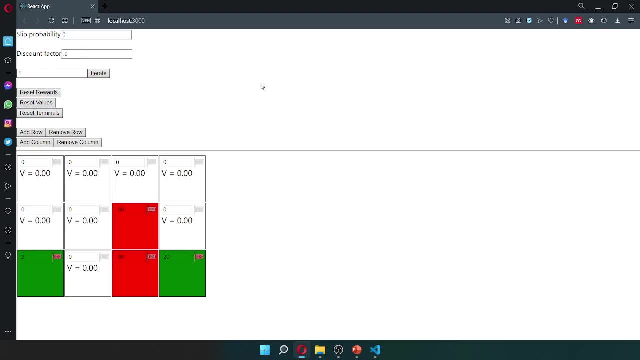 then yeah, let's just say that our discount factor is 0.9. also, by the way, these small squares, these inputs here are the rewards if you reach that state. okay, so, for example, if you let's, just let me try another browser- um, i'm trying to find my. 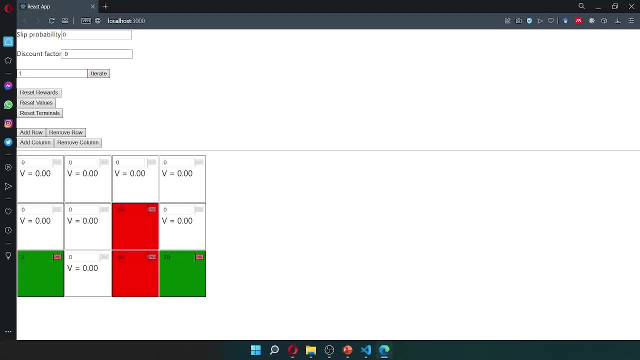 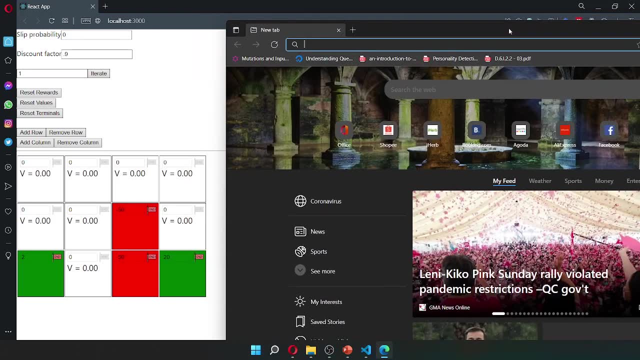 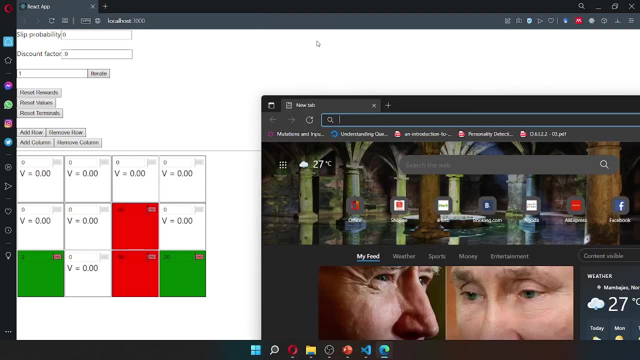 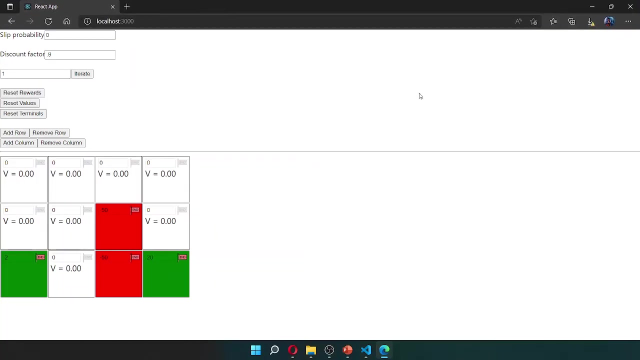 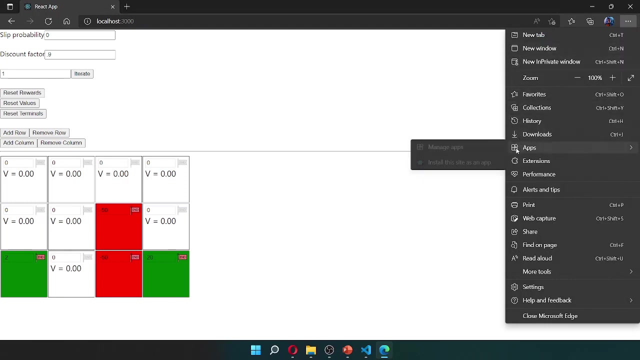 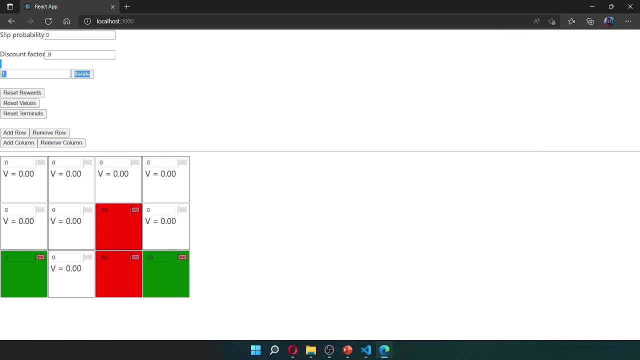 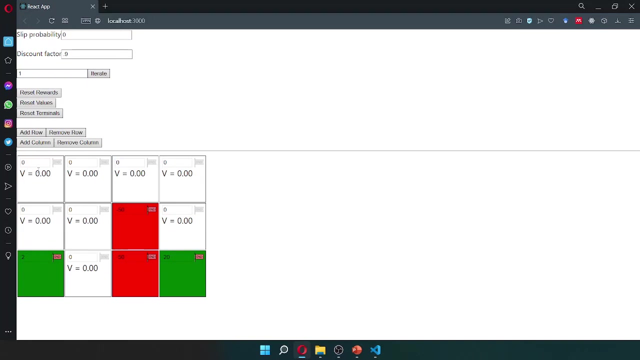 software. i think it is an infinite feature. um, um, you know what? never mind. let's go back to my favorite browser opera. okay, so let's just say that you're in this state, the upper left state, and you and your agent goes down. so, basically, your agent will receive. 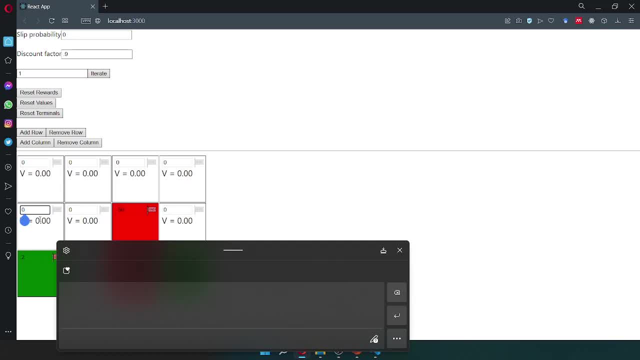 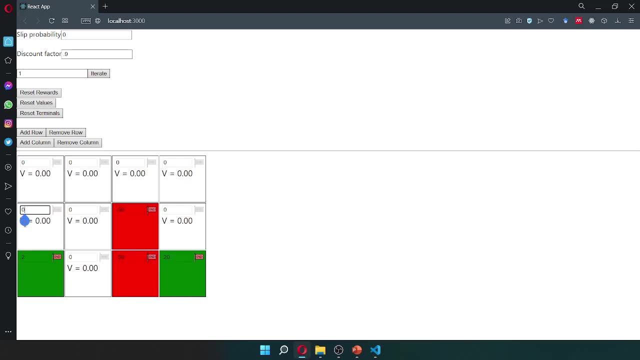 zero reward, okay, okay, what if your agent is this state, okay, this, the one in blue, the- you know you can see here the blue something. so what if your agent is in that state and then it goes down? so after going down, your agent will receive a reward of two and the game will end also. that's just how uh things are represented also. 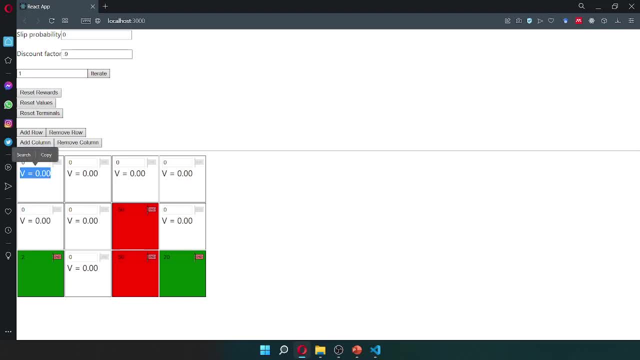 the v. okay, v is equal to something that's, that is the value, that is the value of that state at the current iteration. okay, so now, um, let's try simulating um the values. okay, i mean the value iteration, so i'm, i think, so okay. by the way, the actions that are allowed: 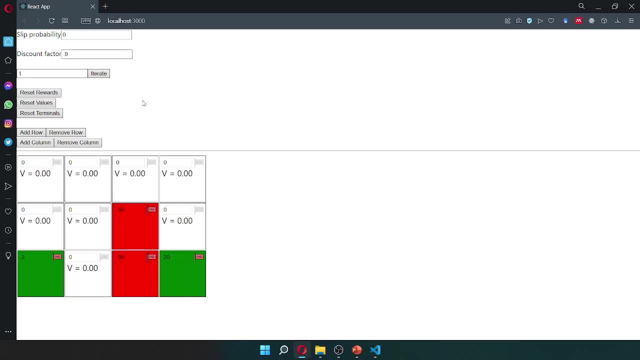 are only up down left, right. if you go to the edge uh, when performing any action, you will just go back to the state that you are in. okay, so if i click iterate, the values should update at t. uh, t is equal to one, okay, so basically, what you're looking at right now is t is. 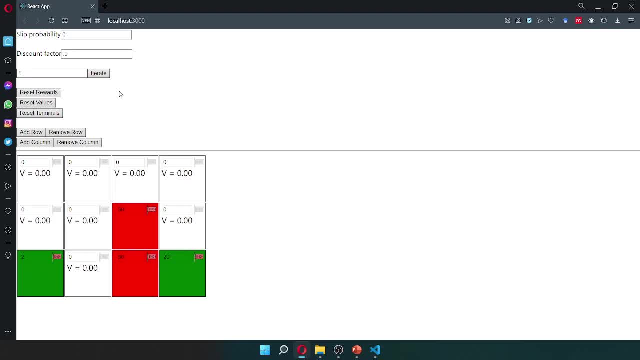 equal to zero. if i click on iterate, we will see t is equal to one. so i i think this will be 20.. this will be 20.. okay, this will be 20.. two and then this will be two. the other things will be zero. okay, iterate okay. 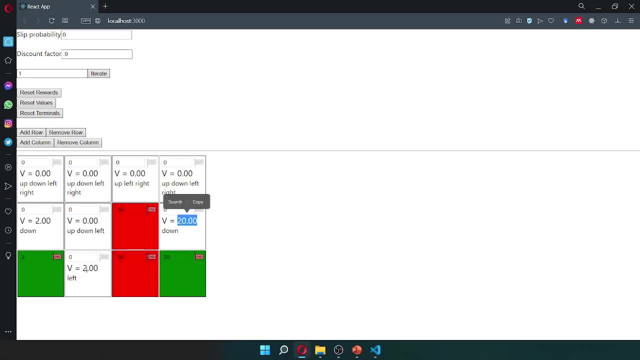 right, so i was correct. this will be 20, this will be 2 and then this is also 2.. also notice: the policy at this state is down. so this tells us that if you are in this state, it is best if you go down also in this state. if you are, if our agent is in this state, it is best if it it goes. 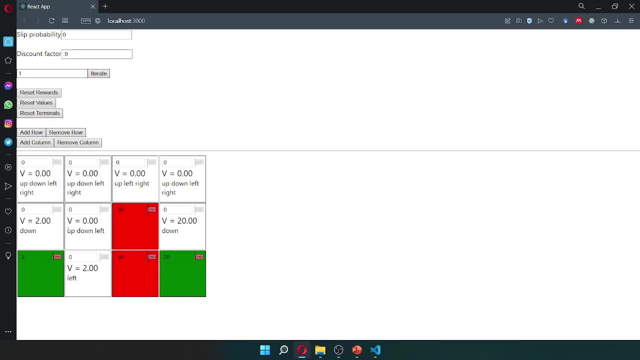 left, okay. however, um, here, uh, the actions are either up up, down or left. so notice that there is no right, because, yeah, the value here is: um, yeah, you don't want to go here because the reward is negative 50. okay, basically, if you go to the 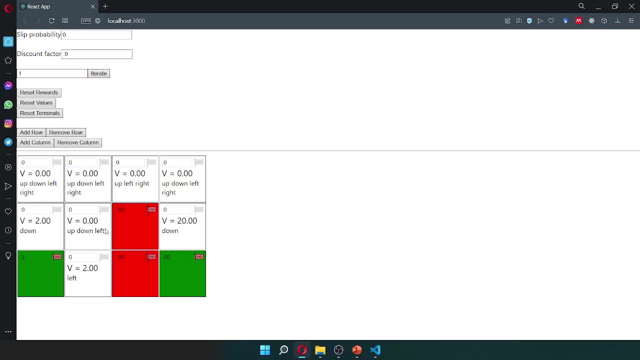 right side, that your, the value will be negative 50.. however, if you go up, down or left, the value of this state will be zero. so that's why, yeah, we have the same values, these actions and the same values. okay, this one, yeah. down if you're in this state. yeah, it's best if you go down, okay. so next. 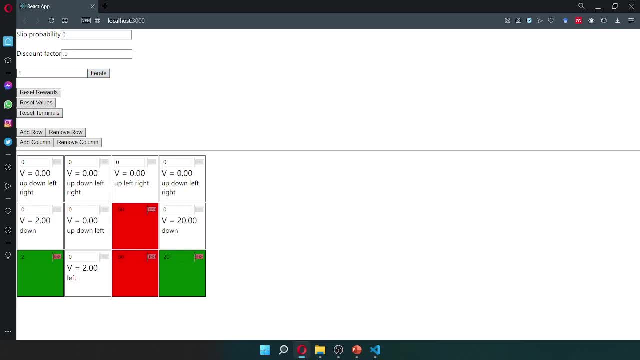 we iterate at 40. to 2.. i'm assuming the value of this will be 20 times 0.9. the value of this will be. the value of this will be 20 times 0.9. the value of this will be. 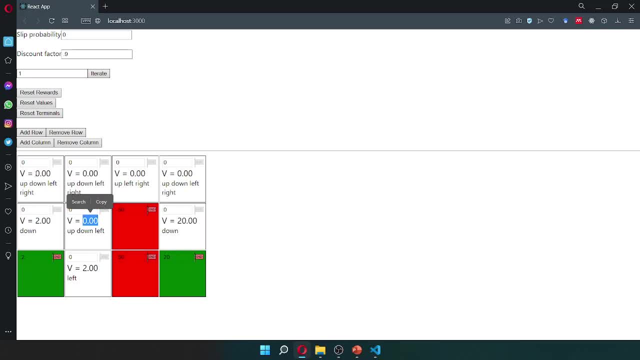 2 times 0.9, so i guess 1.8. is that correct? this will be also 2 times 1 for uh, this also. this will also be 2 times 0.9, which is equal to 1.8. let's see if i am correct. 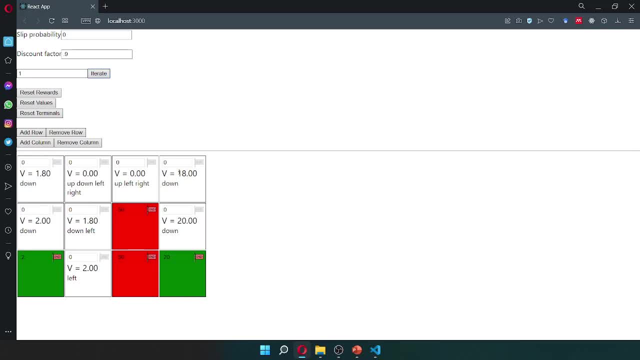 yep, okay, i am correct. you can see here. this is 18, this is 1.8. so notice also that the um, the value, uh, the policy have updated. so, instead of going down and right, this has changed to um just down. so this one, instead of going up down left, this is it the policy at this? 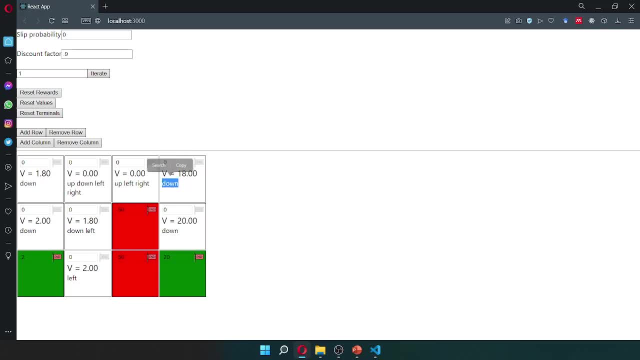 date has changed to just down and that, so this also just changed to your just two down. next, iterate, for t is equal to three. um, i think this will be 18 times 0.9. yeah, this will be 18 times 0.9. this will be 1.8 times 0.9. 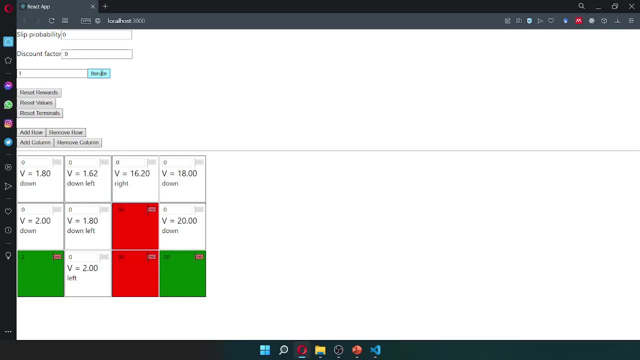 so okay, yep, i was incorrect again. so change to 16.20. this is 1.62. the value here also changed to right. i mean the policy here changed to right. that's, the best action to do when you are here in this state is to go right. however, this is still down and this has changed to down or left. 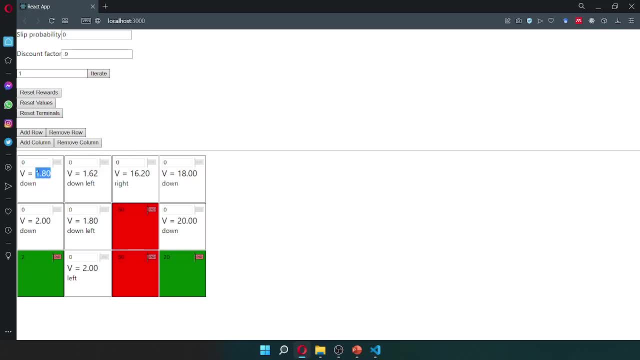 here because, yeah, the values here are equal. so what will happen if we enter it again? so i'm predicting that the value of this will change. okay, the value of this will change to 16.2 times 16.2 times 0.9, and then the policy here will become right. 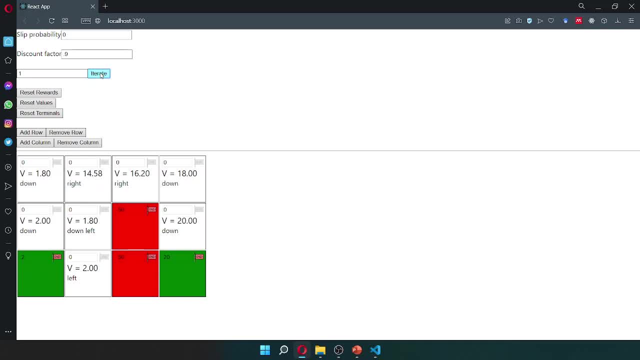 so if we iterate, iterate- Okay, I'll just write again. If we iterate again, if we repeat our iteration, this will become 14.58 times 0.9.. This will become 14.58 times 0.9.. And the policy here? 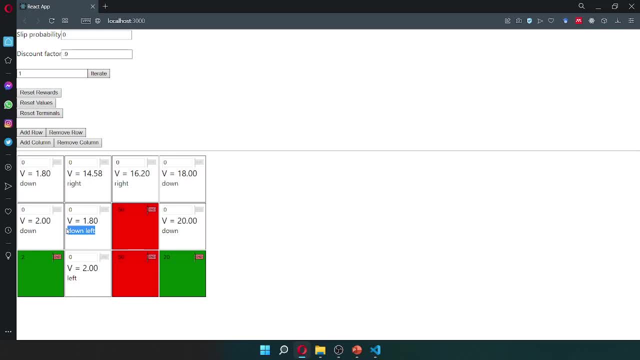 will be right. The policy here will be up. Okay, let's see if I'm correct. Okay, right, and then up Next. How about this one? Okay, so I'm predicting that the value here will be 13.2 times 0.9.. The value here will be 13.2 times 0.9.. And also, the policy will be: 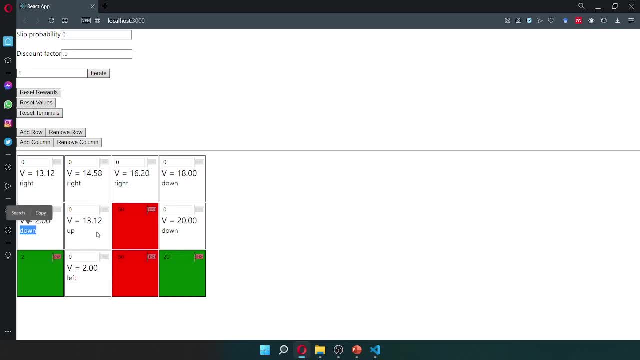 up. The policy here will be, I guess, up and left. No, no, up and right. So iterate, Yep, I'm correct again: 11.81,, 11.81.. Then up, Then this one up and right. So yeah, if. 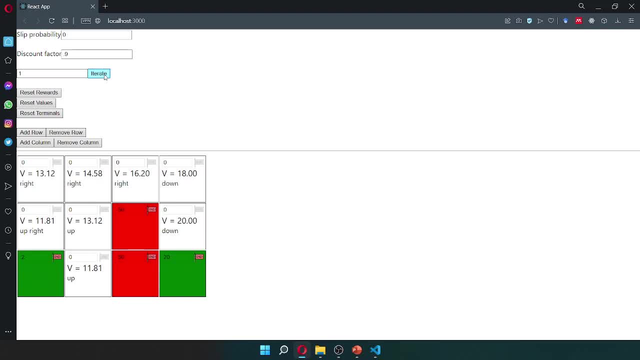 we do our next iteration. nothing happened. Click again: nothing happened, Nothing happened. I'm just clicking, clicking, clicking, Nothing happened. This tells us that we have reached convergence because the values have not changed. So again, we have reached convergence because 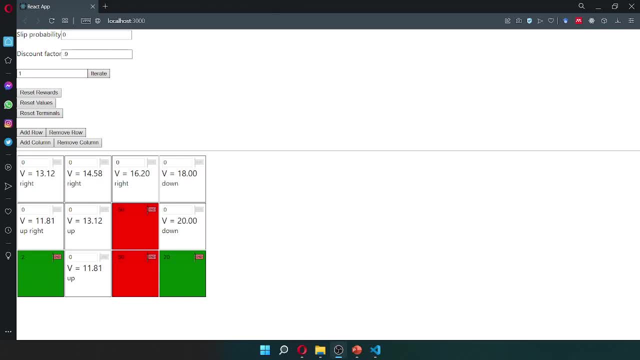 the values have not changed. So yeah, that's just how simple it is: propagating backwards. Okay, so I have reset the board. Okay, so I have reset the board. As you can see, the rewards here have become back to zero, And then the values have also become back to zero. 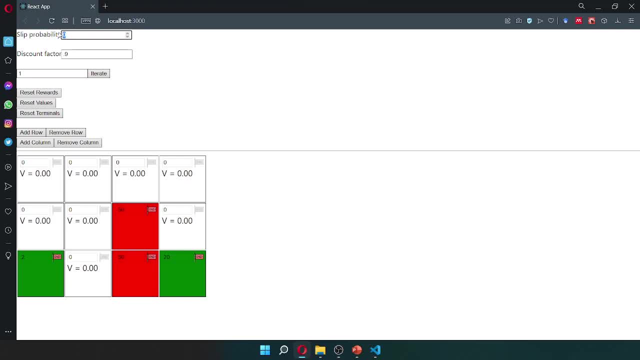 So now let's introduce slip probabilities. so now we will have probabilities. so the slip probability is basically the probability that, um, the agent will take a random action. uh, that is against your current action. okay, so, okay, okay. so, for example, for example, you are in this state, okay, 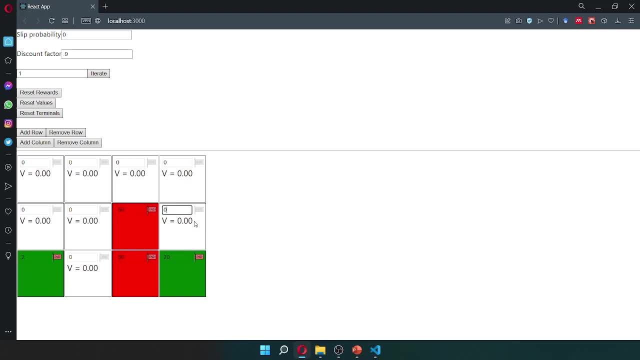 you are in this state and then your agent decides to do, uh, to act or to perform the action down. okay, so if your agent tries to perform the action down, um, there is a, there is a probability that the agent will not go to this state. so there's a probability which we will call the slip probability. 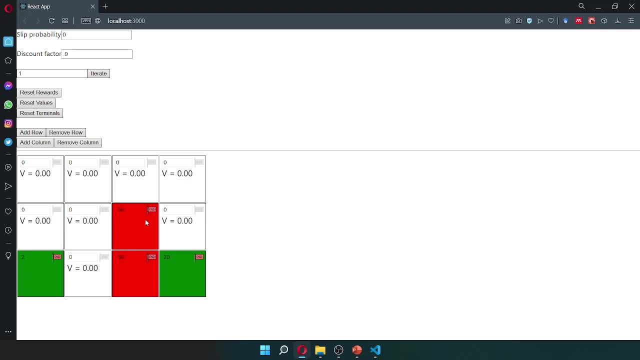 that the agent will instead take um left, right or up. okay, so again. so again. let's assume that you are in this state and your desired state, uh, your desired action is down. okay, your desired action is down. however, um, instead of going down, there's a 0.1 probability that your agent can go to the state. 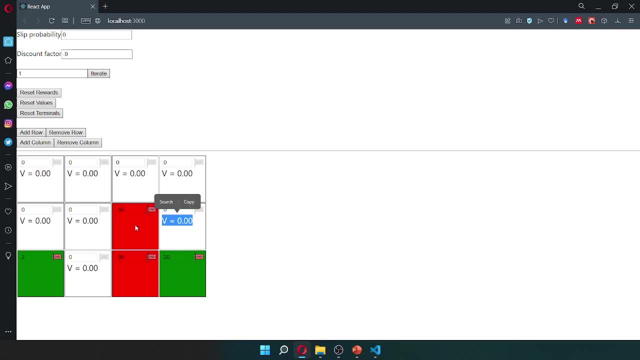 you can go back to this, to this, to the current state, or go to the state on the left or go to the state on the top. okay, so we call that the slip probability. so let's just say that the slip probability is 0.1. so if the slip probability is 0.1, there is a 0.9 percent. uh, there is a 0.9. 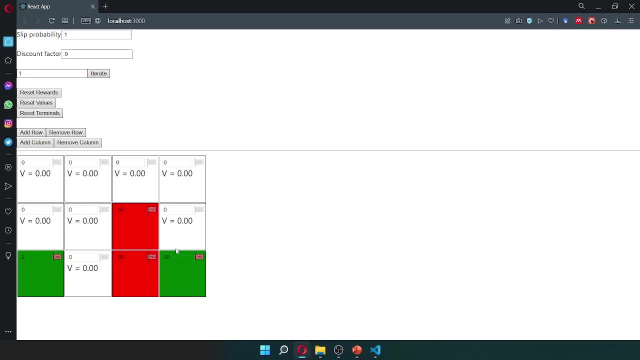 probability that the agent will go down, if you want it to go down. and then there is a 0.1 probability that the agent will go to either left up or the same state, if you want, if they, if you want it to go down, okay, so it's a bit confusing, but yeah, it's a bit confusing, so i'm just gonna repeat one last. 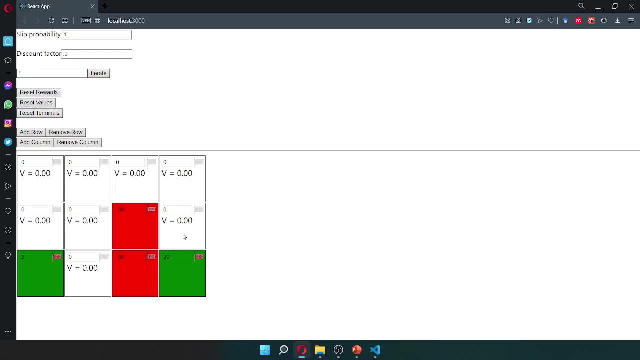 time. so there is a 0.9 probability. so basically, one minus one minus 0.1. okay, there's a 0.9 probability that the agent will go down or, if you decide to go down, and then there is a 0.1 probability that it will either go to the left. 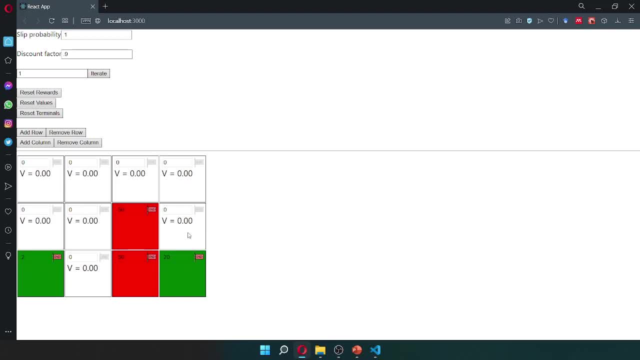 up or the same state. okay, so now let's try to calculate the values with a 0.9, 0.1 slip probability, iterate, iterate, iterate, iterate, iterate. okay, all right, so the values didn't change anymore, right? so it looks like? um, okay, it looks like uh. 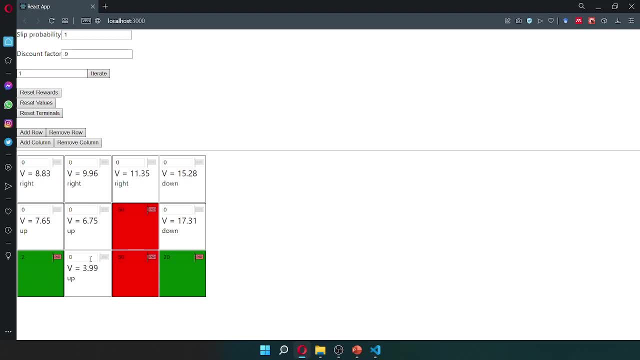 the. the solution to the, to this mdp or this problem, is to go to um, to the reward that has, that has the value of 20.. okay, to the growth state of 20.. so, if you are, okay, so, for example, you are in this state. 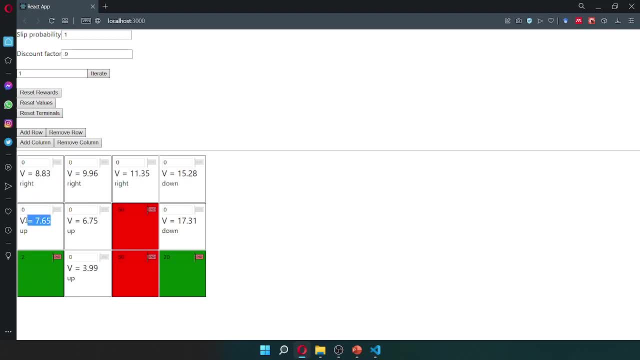 If you are in this state, the agent is being told to go up up right, right, down down. The agent is in this state, it is told to go up right right, down down. If the agent is in this state, up up, up, up right right, down down. 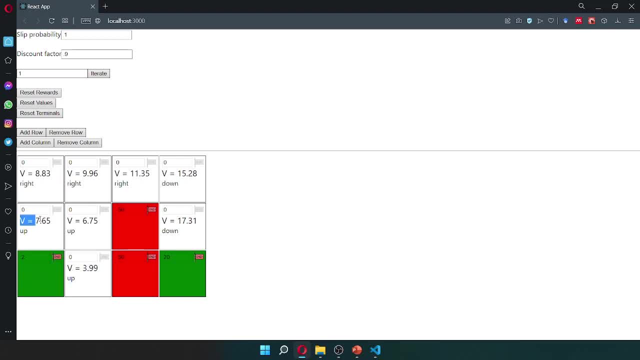 Notice. I want you to notice something. Notice that the agent in this state will go up, only It will not go to the right, Okay. so again, notice that at this state the agent will just go up. We do not have a go, right. 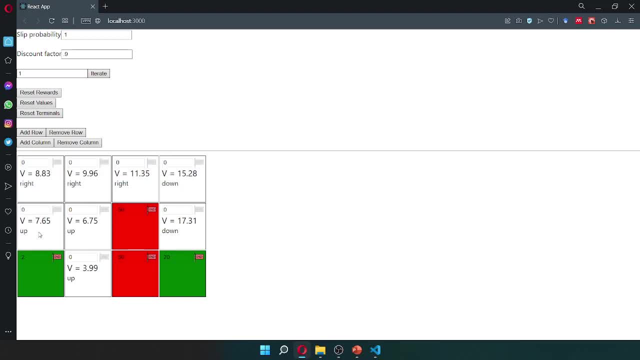 We do not have a go right action here. Okay, It's because if the agent goes to the right, you increase the risk that it will slip into the punishment, So that's a bad thing. So we have just taught our agent to avoid the tiles where it will most likely be punished. 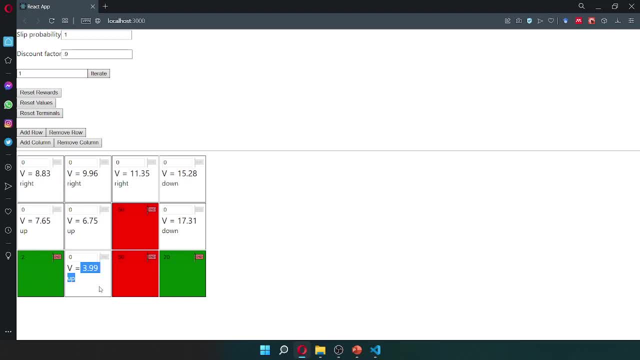 So those tiles are this tile and this tile. Okay, so we have taught our agent to avoid these. However, there is no avoiding this, because this is the only way to arrive at this state. Okay, Okay, so let me reset again. 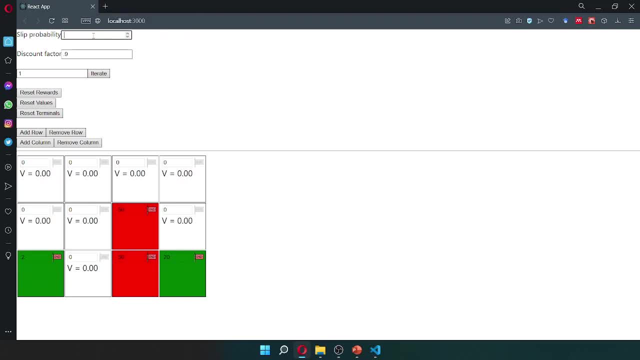 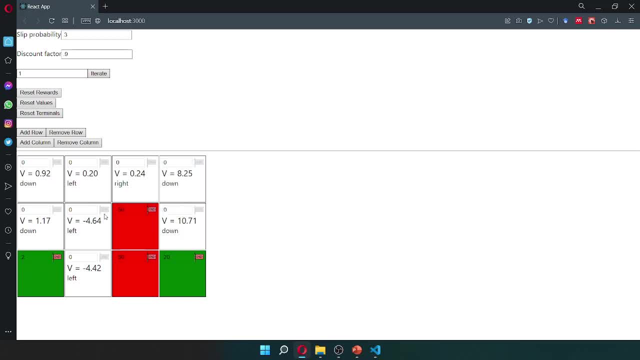 If the agent is in this state, it is also best to go down. Okay, However, if the agent is in this state, it is best to go left, then down and then down. if the agent is in this state, it's best to go left and then down. 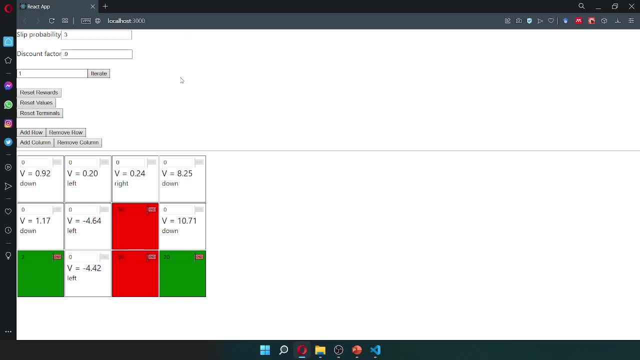 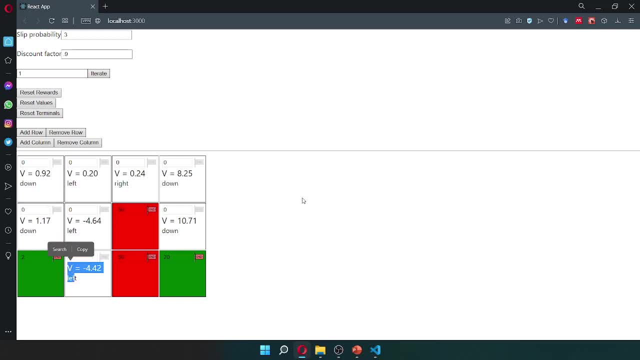 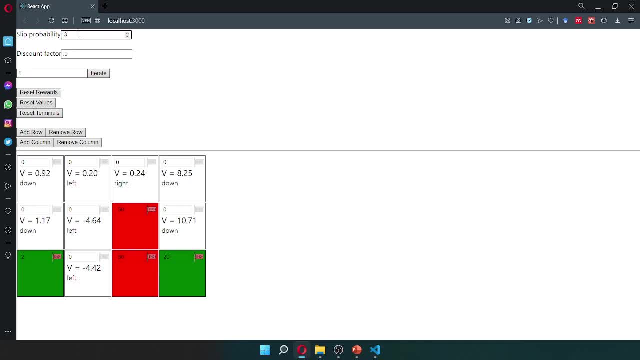 okay, so yeah, let me just finish again. so let's just try the slip probability of um 0.1 again. so let's just go back and then change the discount factor to 0.5. yeah, i'm just curious what will happen. let's iterate, iterate. 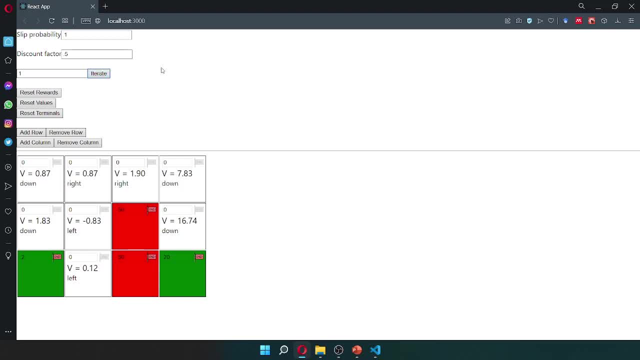 oh, interesting, okay, it's interesting. so, now that the discount factor is smaller, um, these states, okay, this state, this state, this state and this state will go to the reward of 20.. however, this state, this state, this state and this state will go to the reward of um two. 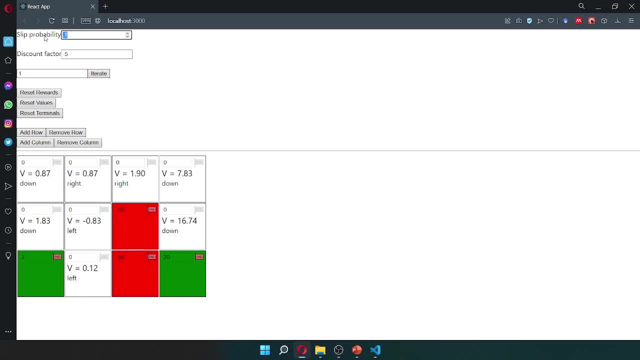 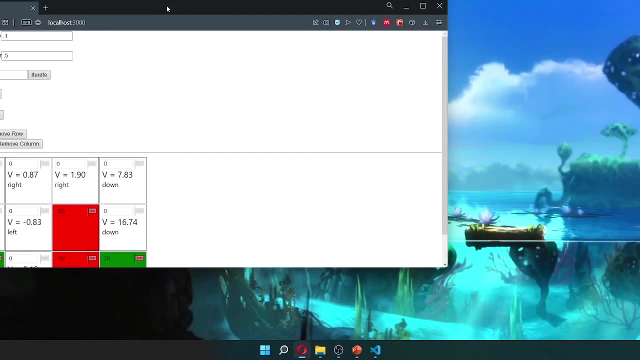 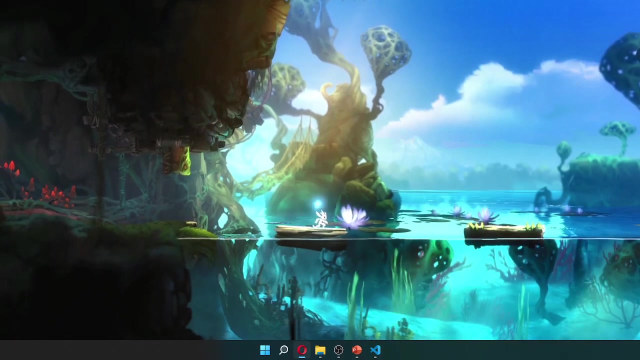 very interesting, nice, oh, yeah, okay, so that's all. i guess. i'm not going to give, uh, any other examples. i think it's enough. so, yeah, thank you. yeah, it's very interesting. these things are very interesting. okay, so let me show you another thing for a while. this is a youtube video that i like about. yeah,